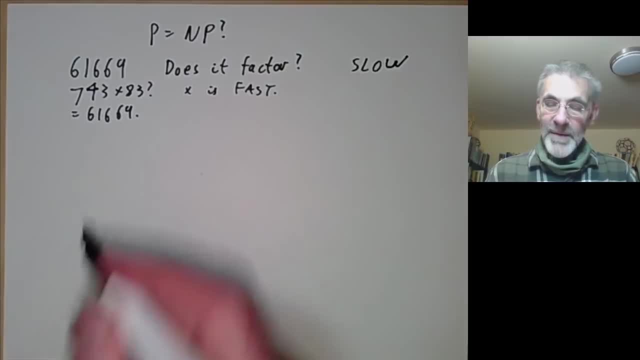 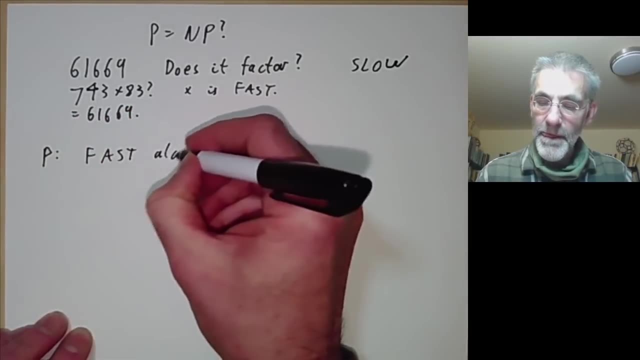 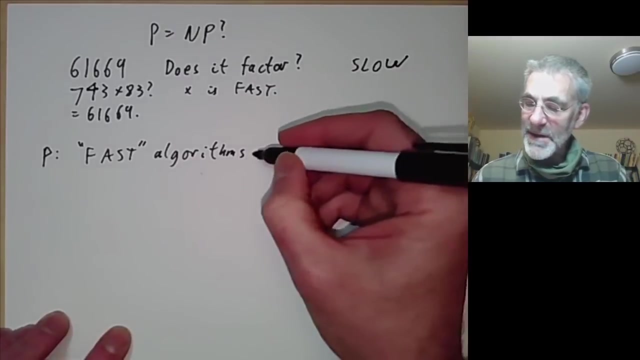 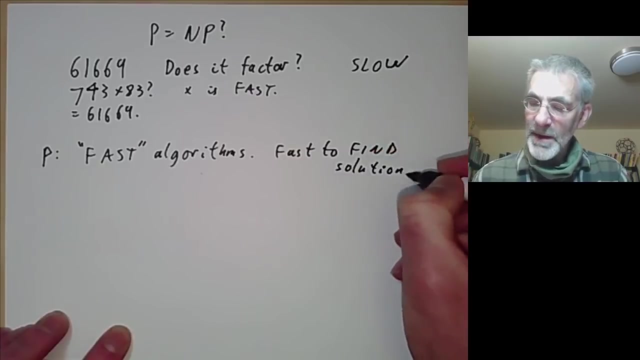 that it is a factorization. And now P stands for algorithms that are fast, roughly speaking. So this is not actually correct. so I'll put this in inverted commas. So that means it is fast to find a solution to a problem. So for example: 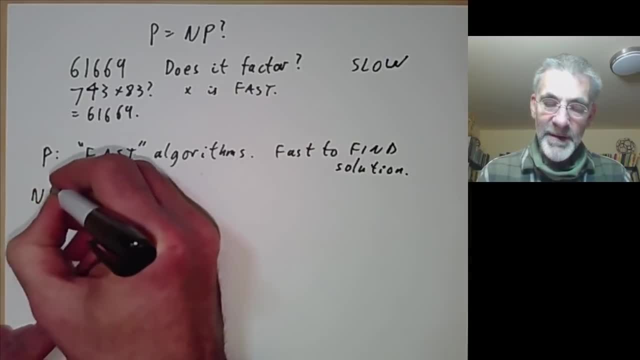 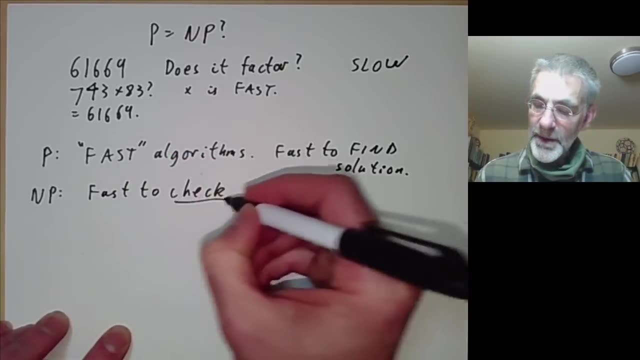 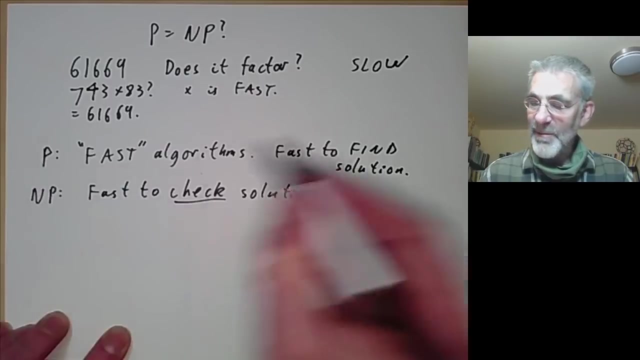 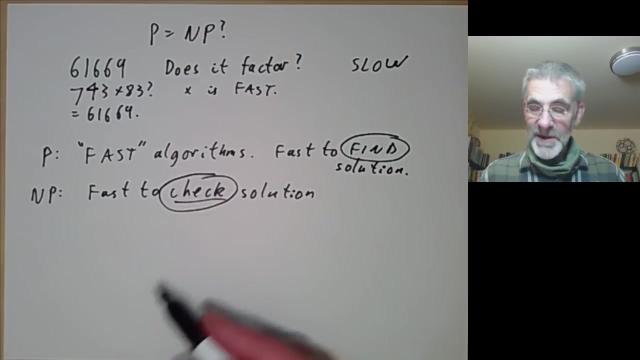 multiplication is fast. On the other hand, NP. we will see that it is fast to check that a solution once you've found one. So the difference between P and NP is the difference between finding a solution and And checking that there's a solution that somebody else has come up with is in fact correct. 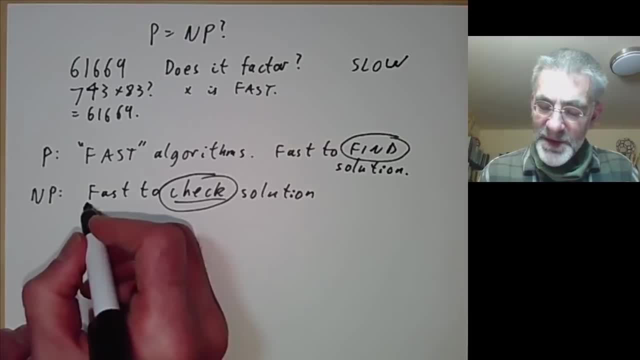 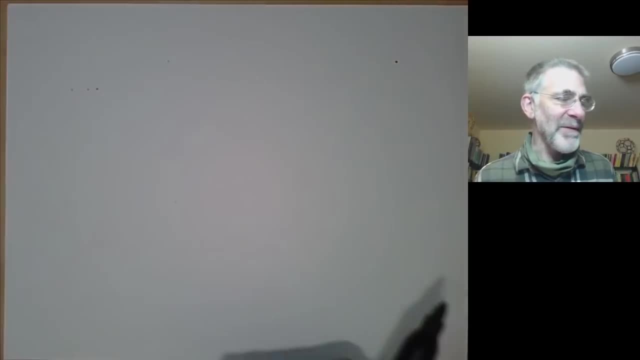 Well, the problem here is- I've used this word fast And the question is, what does fast mean for algorithms? And we want a sort of general definition that doesn't depend on what sort of computer you're using. I mean, it shouldn't depend on whether you're using a pencil and paper. 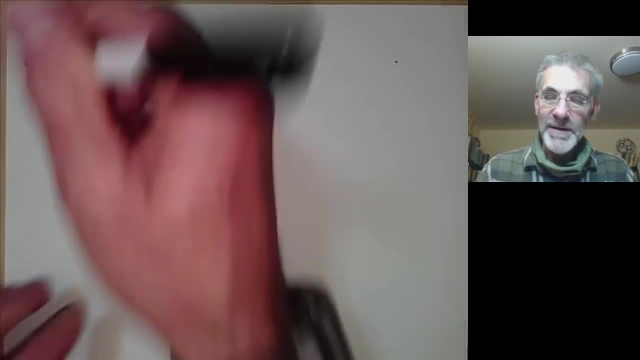 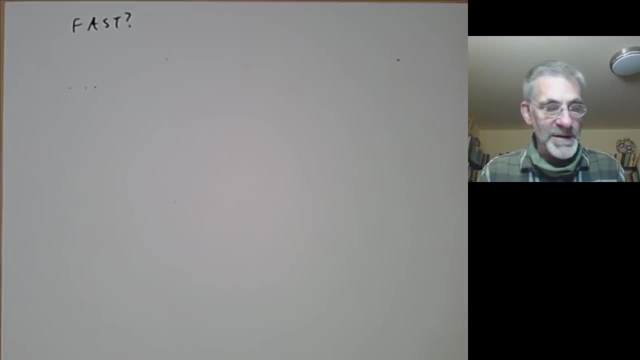 or a computer that can do a billion operations a second. So what's the definition of fast? Well, there's no very precise definition of fast, but there's a reasonable substitute for it, which is due to Cobham, who came up with this in the mid-60s. 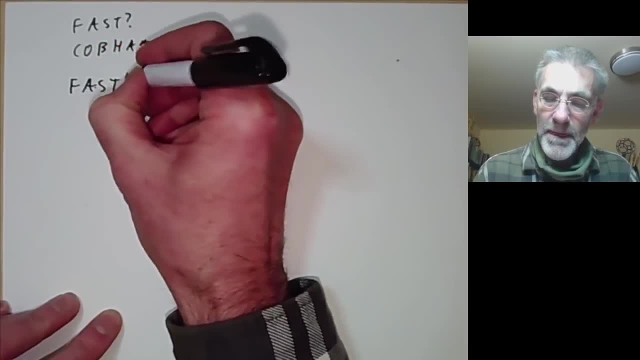 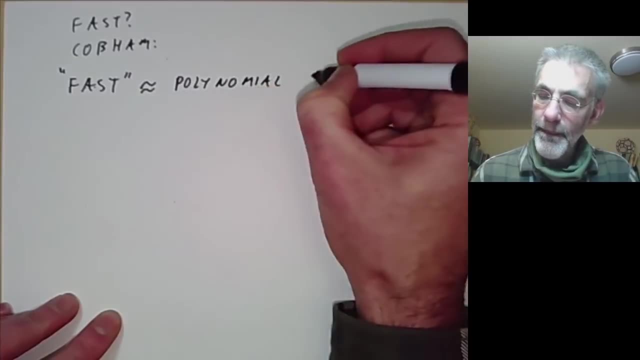 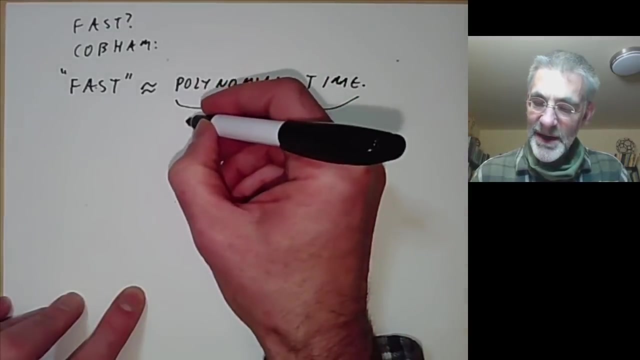 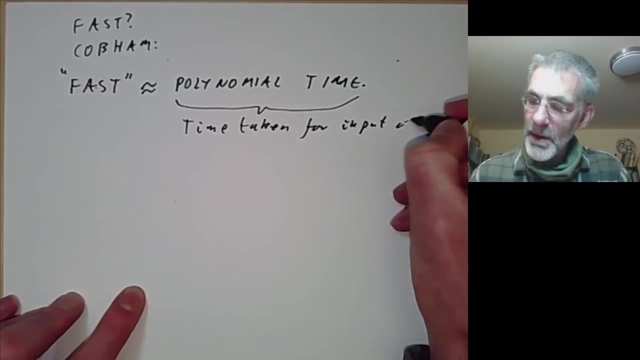 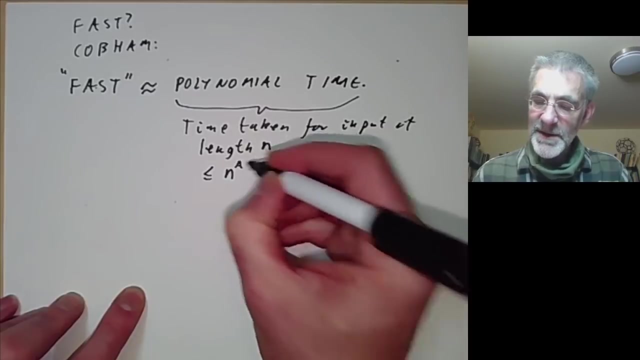 which says that fast for algorithms is roughly equivalent to polynomial time. So So let me explain what this means. Well, polynomial time means the time taken for an input of length. n should be less than or equal to some polynomial in n, such as n to the a for some constant a. 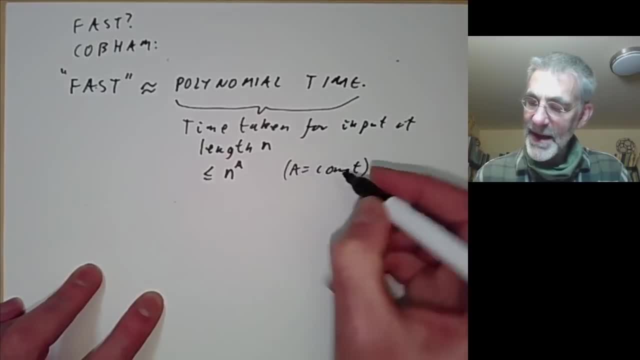 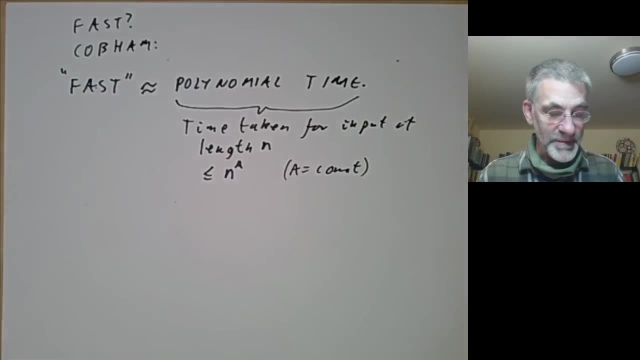 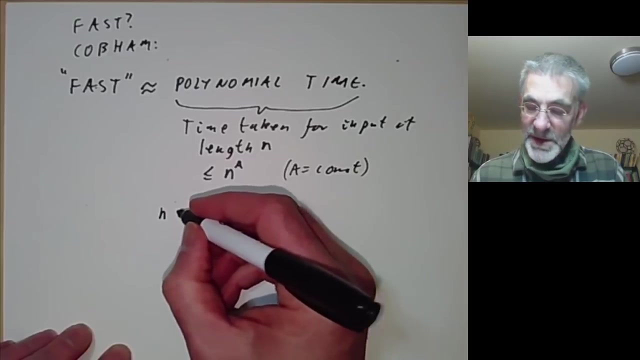 So a is some constant And n is the length of the input And the time should be at most might be at most n squared Or n cubed or something You notice that n is the length of the input. So if our input is, say, 743 times 83,. 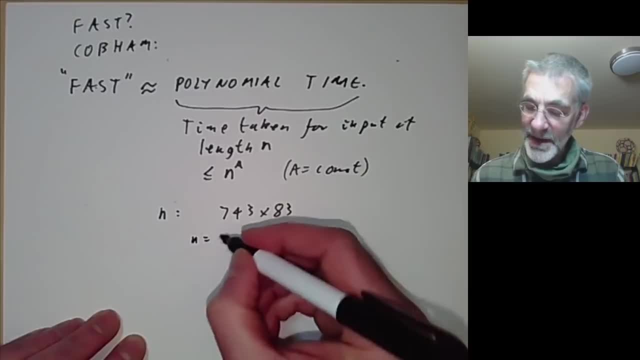 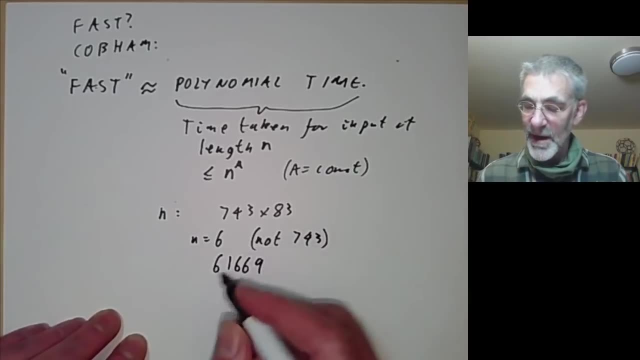 then n is equal to 1,, 2,, 3,, 4,, 5, 6,, not 743.. And similarly, if we were factorizing 61669, we don't want to factorize it in time- that's polynomial in 6169. 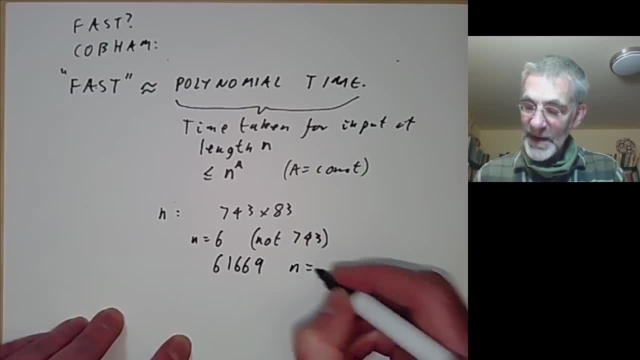 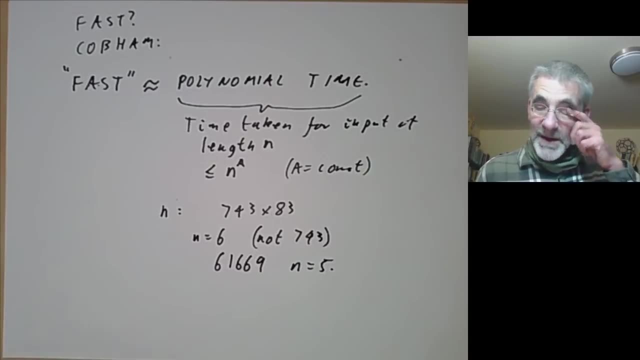 Which would be really easy, But we want to factorize it as a polynomial in the number of digits, which is 5, which is very much harder to do. So fast algorithms roughly correspond to polynomial time algorithms, But you can find plenty of counterexamples. 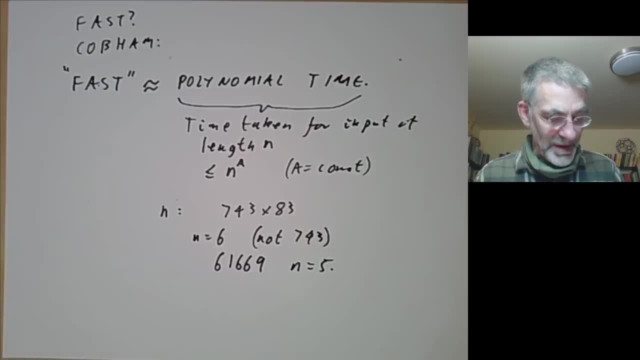 For example, the simplex algorithm in linear optimization is a pretty fast algorithm In theory. it's not polynomial time because there are some very, very rare cases when it takes a very, very long time. But these cases are so rare that in practice it's a fast algorithm, although it's not polynomial time. 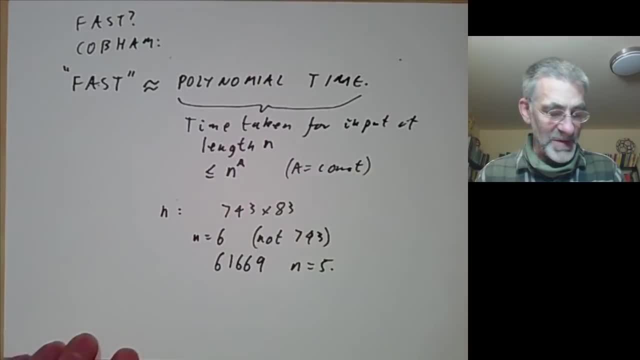 On the other hand, you can also come up with polynomial time algorithms that are not fast. If your algorithm takes n to the power of 100 steps, then that's polynomial time, But if n is 10, this time will be so long that it's not polynomial time. 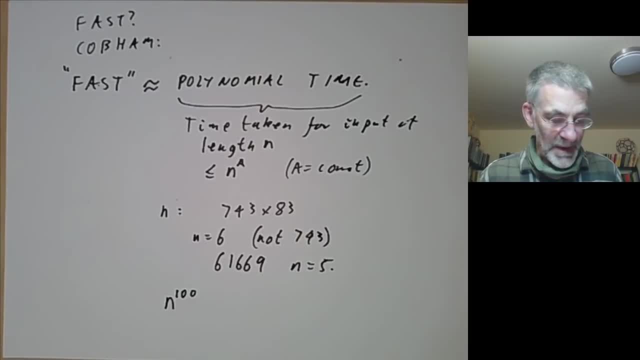 That it's absolutely useless. So, for example, if we do multiplication, this is polynomial time, Because if we take two numbers of, if we take an n-digit number times an n-digit number, the obvious algorithm that people may or may not still learn in high school takes about n squared steps. 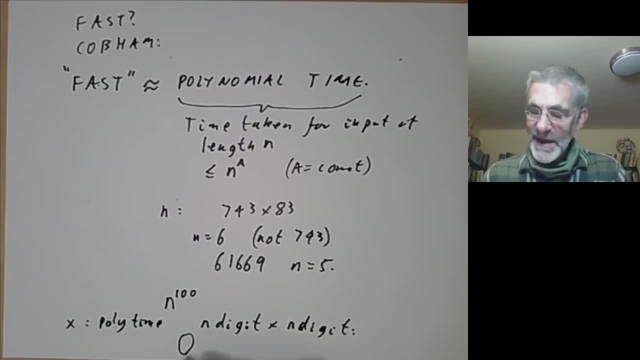 Well, it's difficult to say exactly how long, How many steps it takes. So we say it takes o n squared steps, where o means it's at most a constant, times n squared, And we can't be bothered to work out what this constant is. 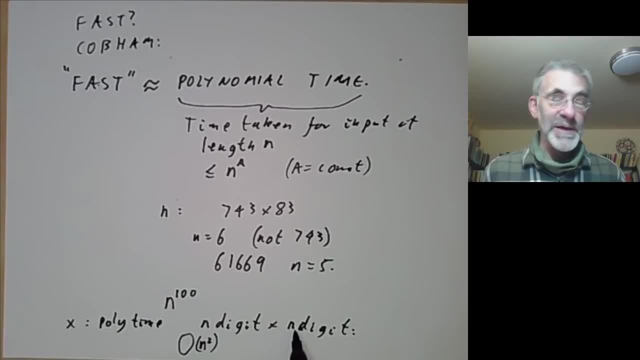 Actually, slightly surprisingly for such an easy and well-known algorithm, this is not the best algorithm for multiplying two numbers. in general. There's a faster algorithm using the fast Fourier transform that takes about o n to the 1 plus epsilon steps, where epsilon is as small as you like. 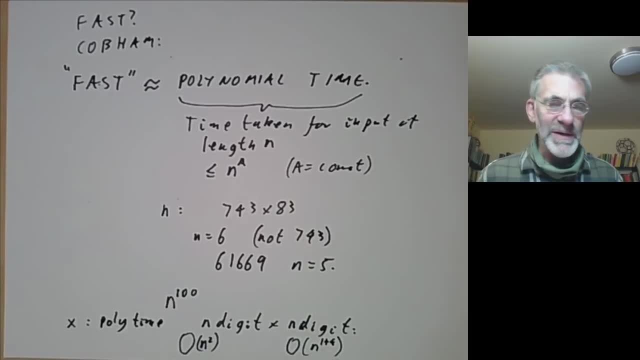 All these numbers like n squared and n to the 1 plus epsilon shouldn't be taken too seriously, because the actual amount of time your algorithm takes depends on all sorts of things like details of the hardware of your computer and so on. So there are always extra factors of powers of log n and so on that people don't really bother putting in here. 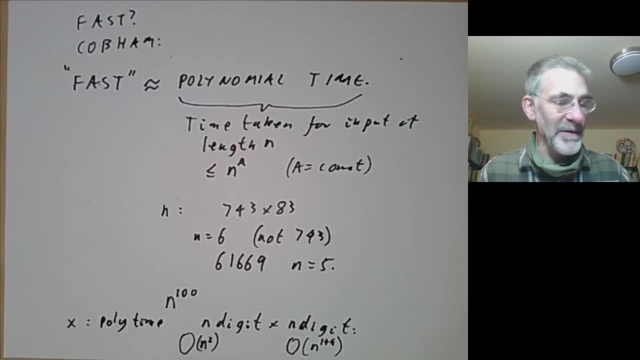 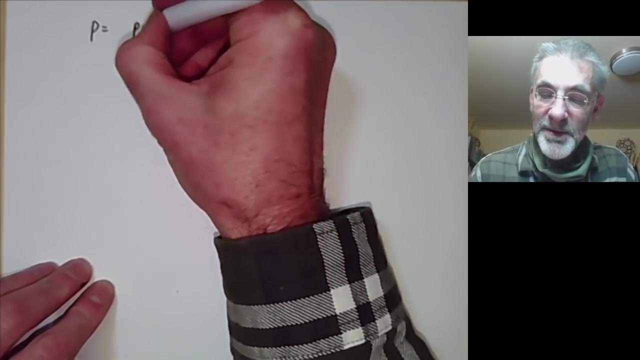 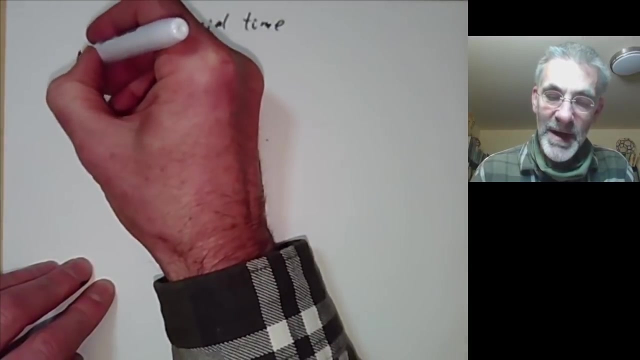 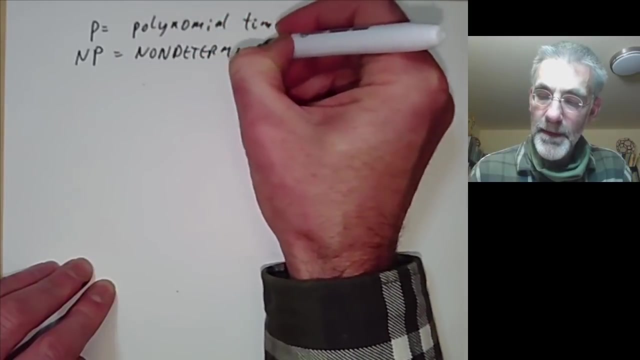 So you should take all these expressions with a bit of a grain of salt. So polynomial time is usually denoted by p, So p is polynomial time, meaning you can solve the algorithm in polynomial time. np stands for non-deterministic, which they've chosen a shorter word. 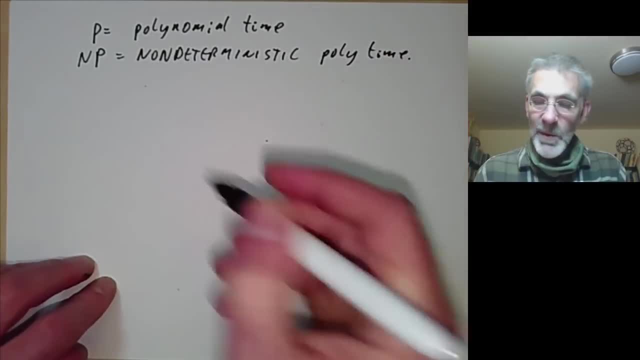 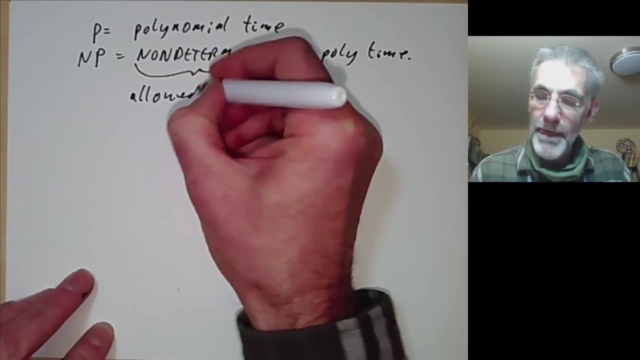 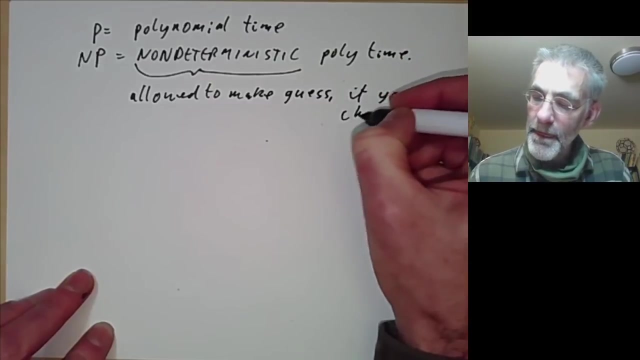 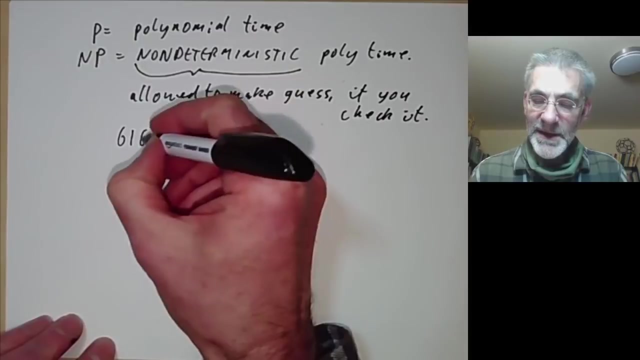 So what does this mean? Well, this means you're allowed to make an inspired guess if you check it. So, for example, a non-deterministic algorithm for factorising 61669 might go like this: You look at your daily horoscope in the newspaper. 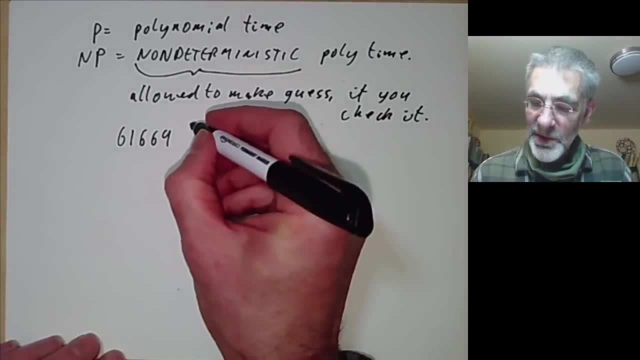 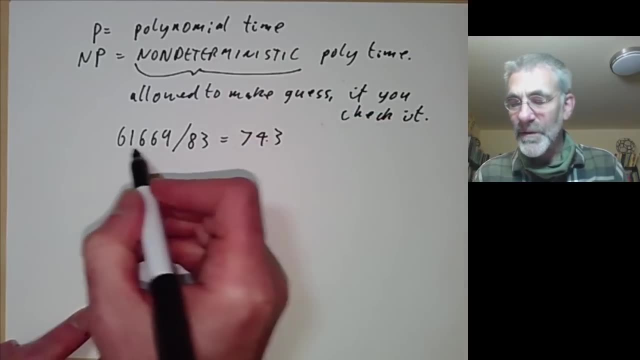 And your horoscope says: well, your lucky number is 83. So you divide 61669 by 83 and you find the answer is 743.. And you can do this division in polynomial time and that checks that the answer is correct. 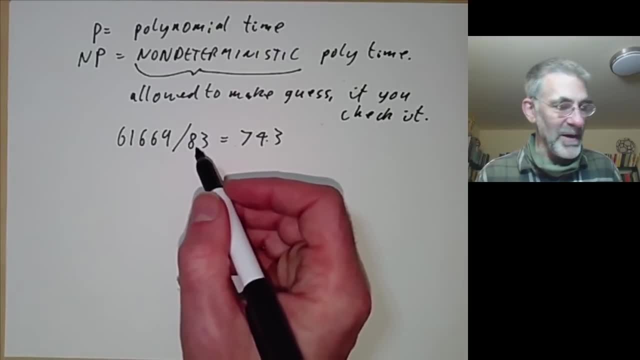 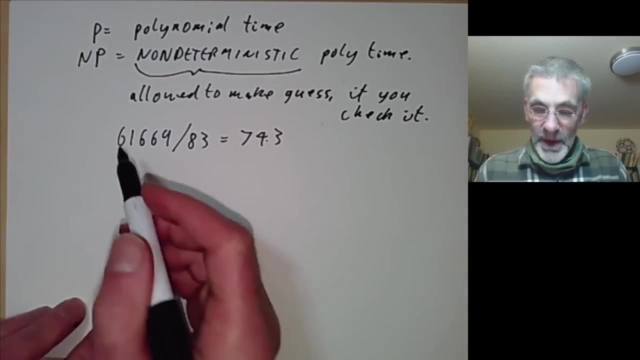 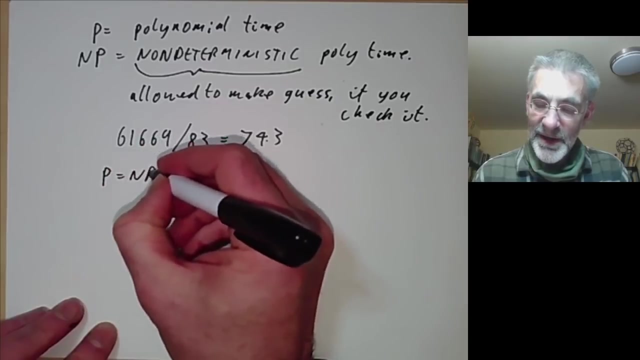 which is probably a good idea, because I don't think astrology columns are really a particularly reliable source of information. So the main question is: the question is: is p equal to np? So if you can solve a problem in non-deterministic polynomial time by making inspired guesses, 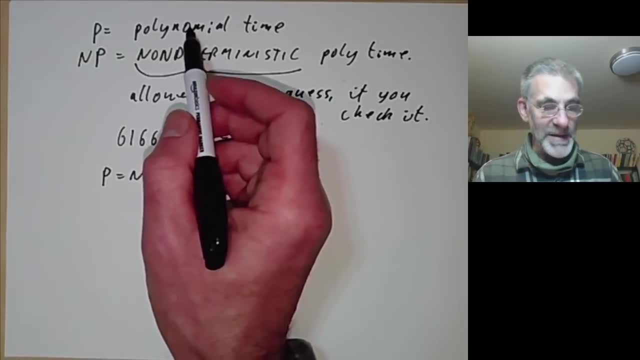 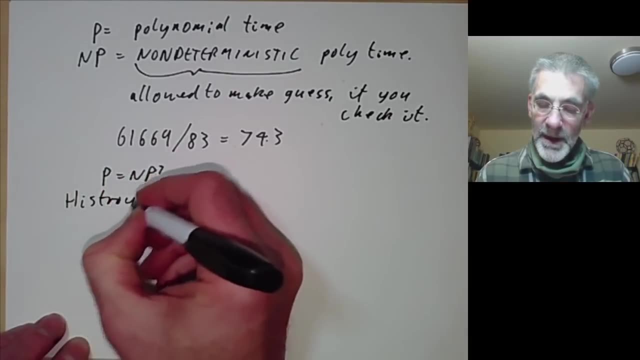 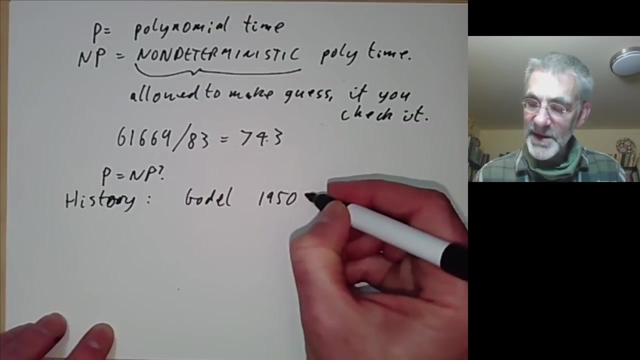 is there an honest way of solving it in polynomial time without needing inspired guesses? So I'll just give the history very briefly. The first person who asked such a question may have been Gödel in about the 1950s, And he wrote a letter where he sort of asked: you know, suppose you've got a mathematical theorem of length. 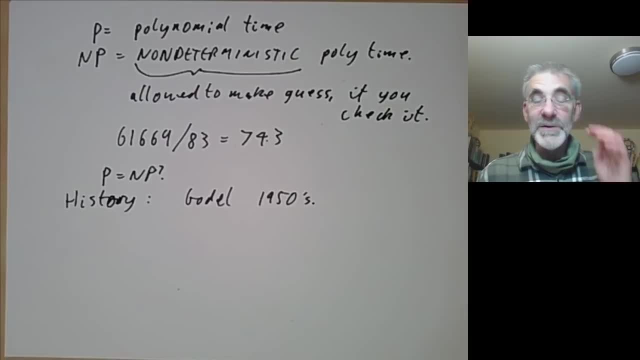 Mathematical theorem: Can you test whether it's got a proof of length n in a time that's linear or quadratic in n or something like that? So he was asking: can you find a proof of length n in polynomial time? And he didn't really push this much further. 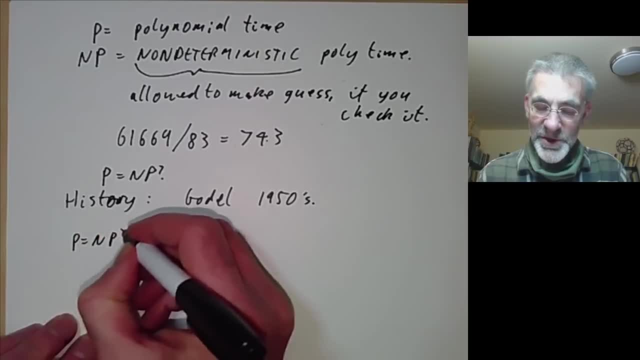 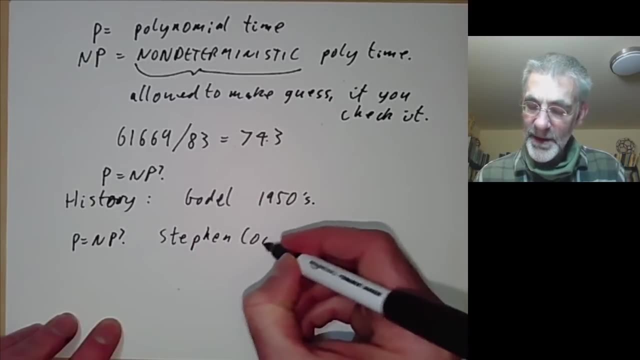 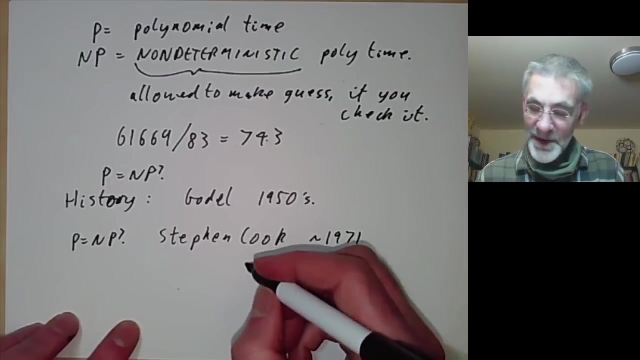 And the p equals np question. it's usually really dated to an article written by Stephen Cook in about 19, in the early 1970s, maybe 1971. And the notion of np completeness and the p equals np question was soon after expanded by Karp. 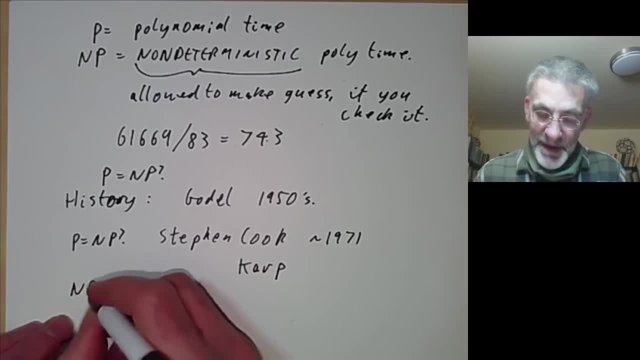 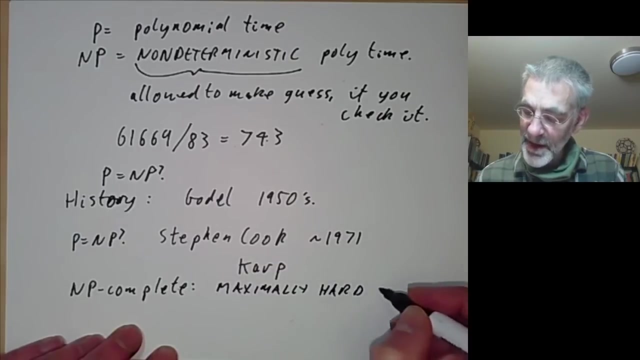 So, in particular, they introduced the notion of being np complete. So an np complete problem is a maximally difficult, maximally hard np problem. What this means is that if you can solve it, you can solve all others. By solve I mean solving polynomial times. 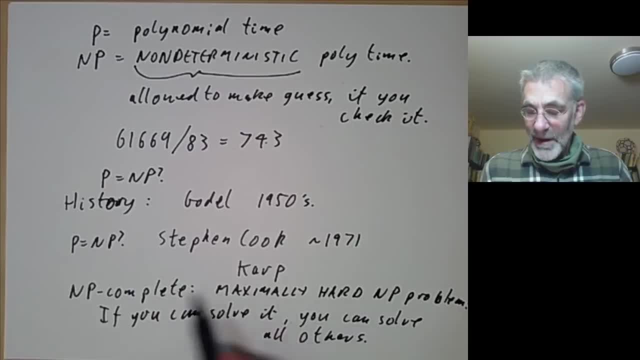 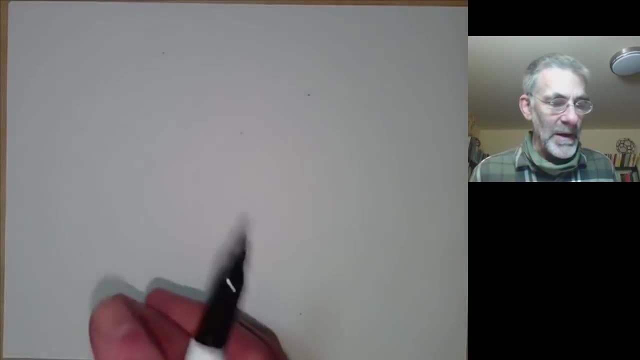 So the question is: so, in order to answer whether np is equal to p, all you've got to do is to show that one np complete problem can be solved in polynomial time. So let's see some examples of this. So first of all, let's ask: 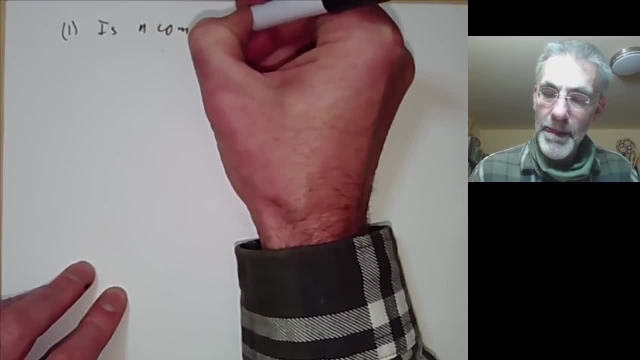 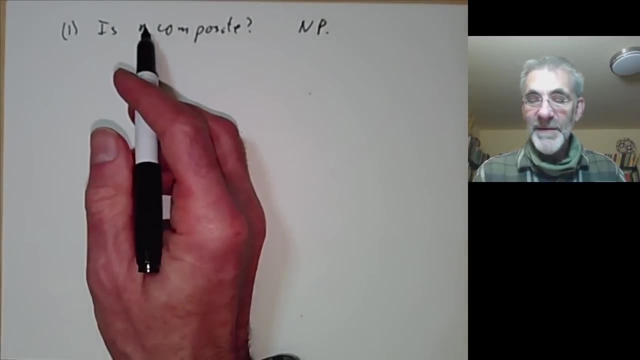 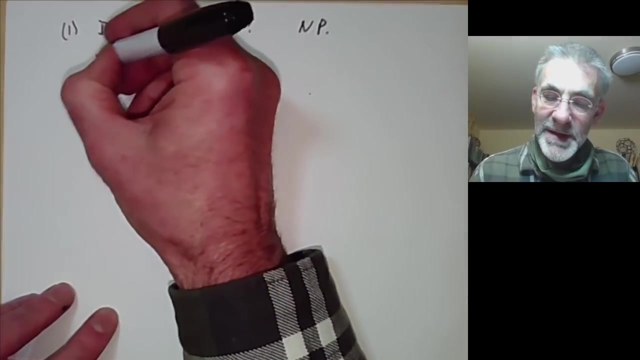 is n composite? Well, this is certainly a nondeterministic polynomial problem, because we've just seen if it's composite, you can make a guess for the answer and check it's correct. Then we can ask: is: is it in p? 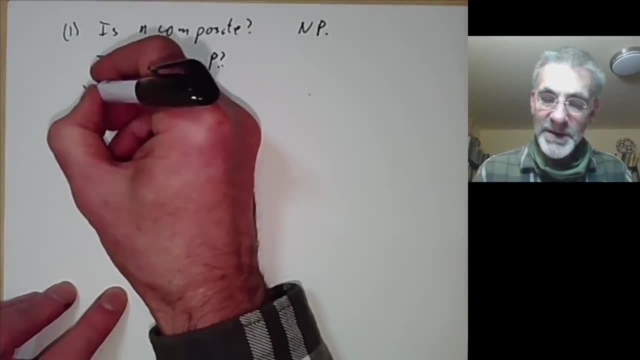 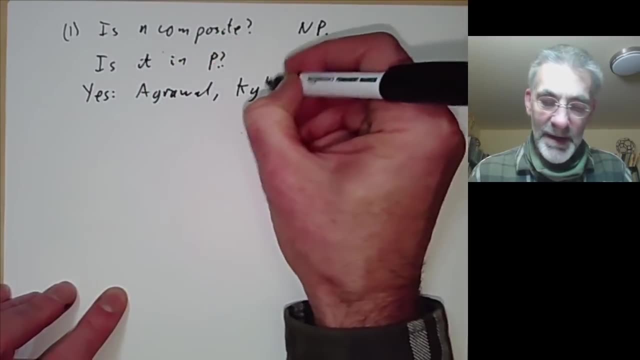 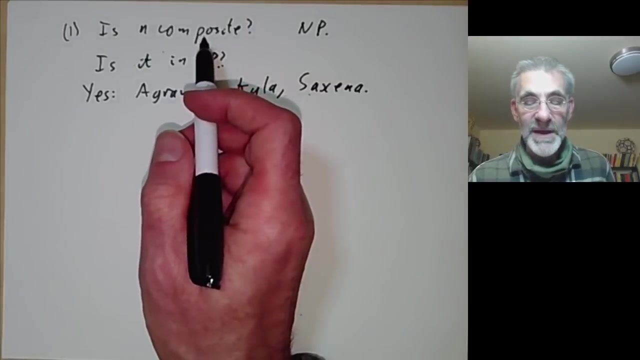 Can we do it in polynomial time without guessing? And the answer is yes, And this was first proved by Agrawal, Kaila and Saxena, who found an algorithm to test whether a number was prime or composite, and they were able to prove that algorithm could do it in polynomial time. 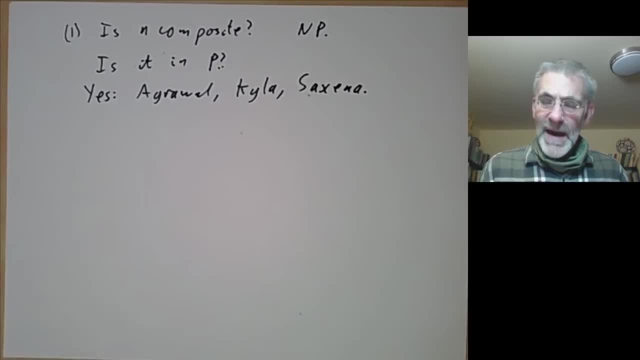 Incidentally, their algorithm probably wasn't the first algorithm that would test numbers in polynomial time. It was the first algorithm for which they could prove that it did it in polynomial time. There were some other known algorithms that probably factor in polynomial time, but the trouble is proving they factor in polynomial time. 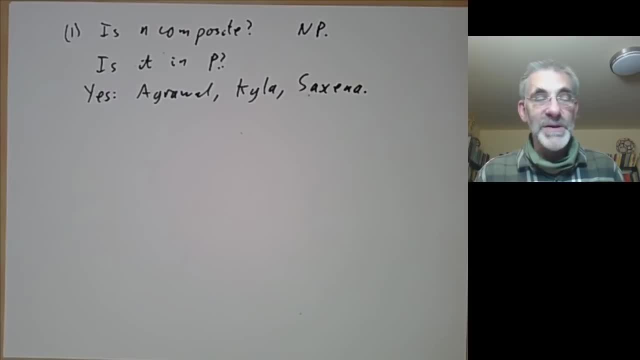 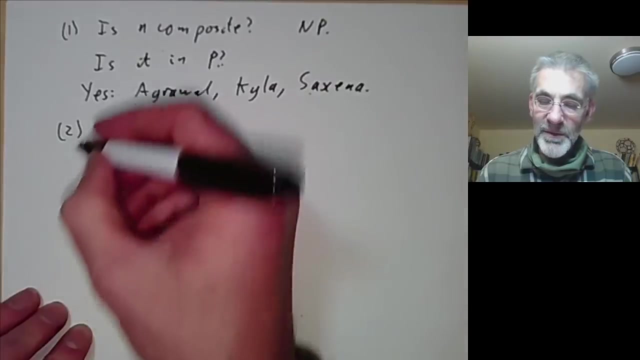 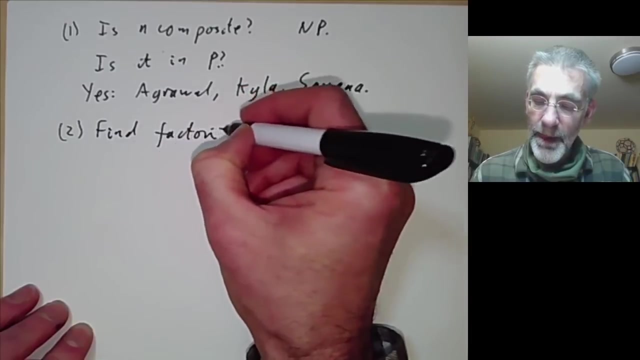 requires using some unproved hypotheses, such as the generalized Riemann hypothesis. So telling whether or not a problem is in polynomial time can be really tricky and difficult to decide. Another example is: well, we first asked: is n composite? We can ask a second question: find a factorization of n. 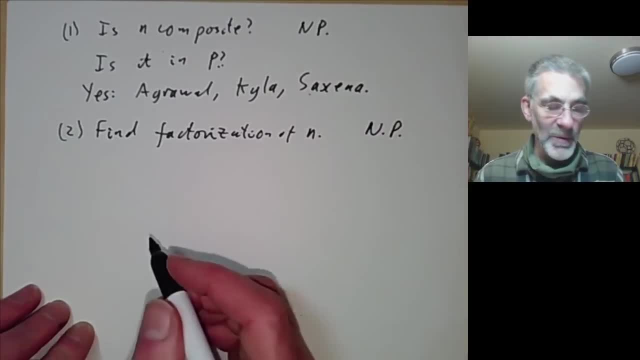 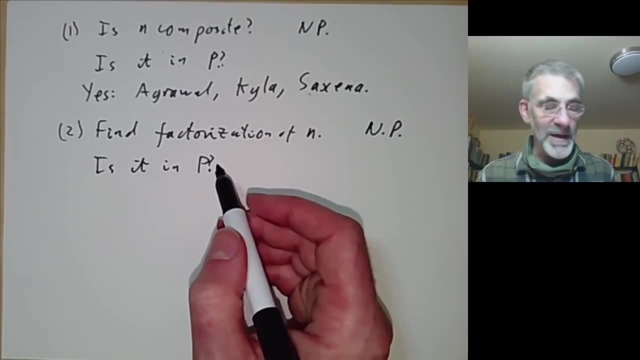 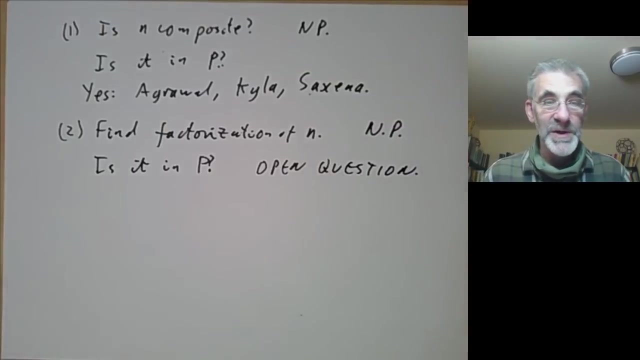 And again, this is a nondeterministic polynomial question and we can ask: is it in p? Can we find a factorization in polynomial time? And this is a completely open question. It's one of the fundamental questions in computational number theory. And I'm not even sure which way I would guess for the answer. On the one hand, people have searched really hard for fast factorization algorithms and never found a polynomial time one. On the other hand, the algorithms are getting better and better. and there are all sorts of really deep ideas that we haven't yet used, so I have no idea whether the answer to this is yes or no. Notice, by the way, that the algorithms to test whether n is composite, the fast algorithms, don't do it by actually finding a factorization of n. 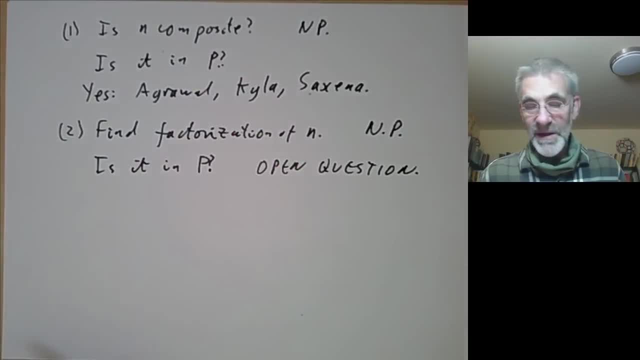 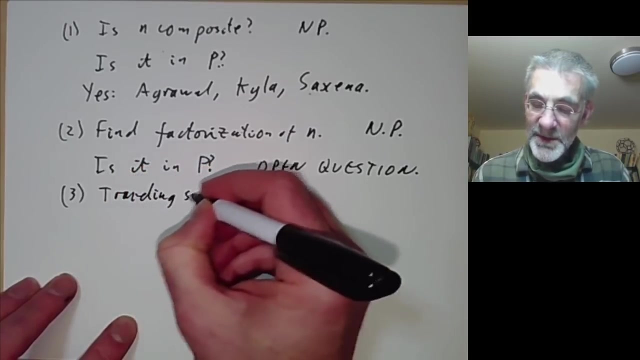 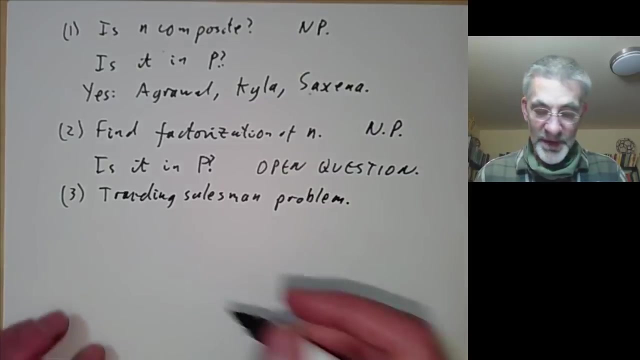 They do it by rather more subtle means. Go and see a course on number theory if you want to know how. So now I want to give an example of an NP-complete problem. The classical example of this is the travelling salesman problem, Salesperson or whatever. 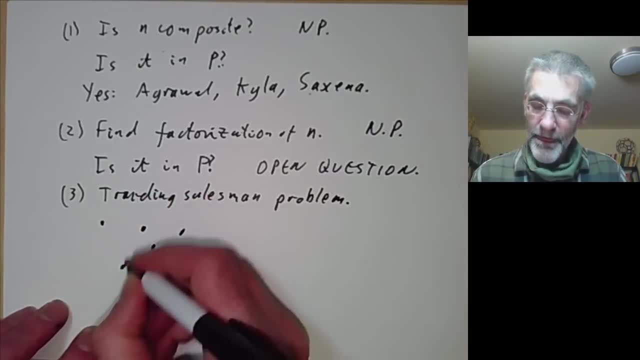 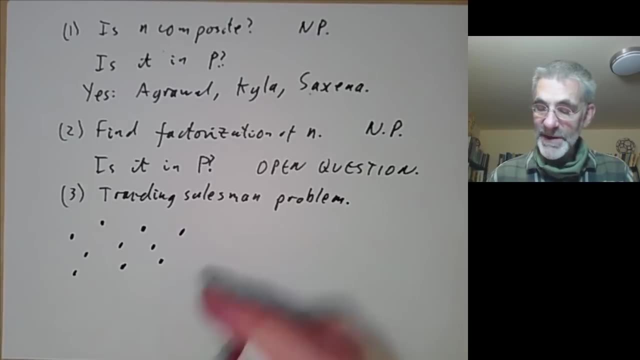 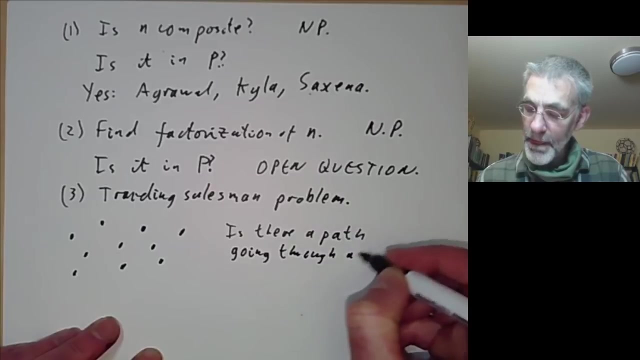 So this problem says: suppose you've got various towns And a salesman wants to visit all these towns in the shortest possible way. So we ask the following question: Is there a path um going through all the towns of length less than or equal to k? 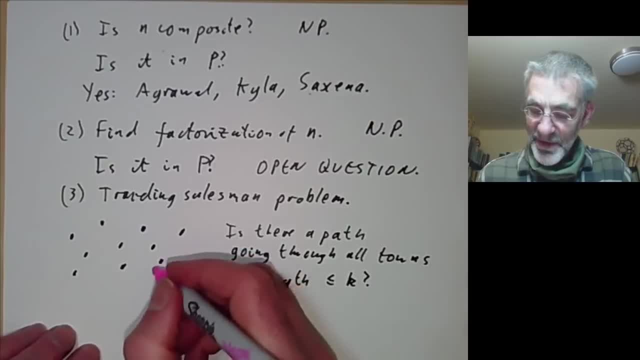 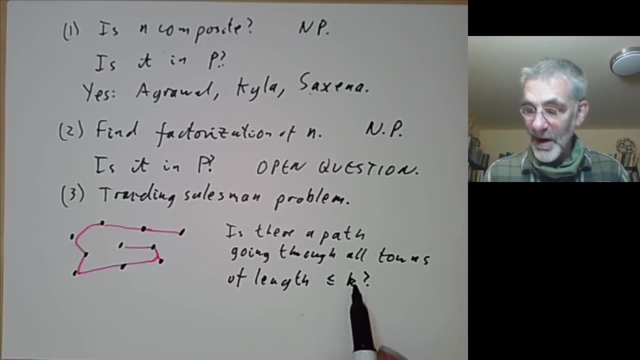 So you might sort of guess that a path is going to go around like this. So this might be a reasonable candidate for the shortest path. And this is obviously a non-deterministic polynomial, because if there's a path of length less than or equal to k. 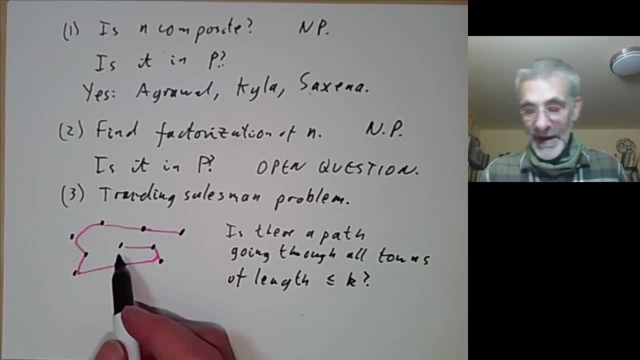 you can just write down the path and check it's got length at most k And you can sort of. that basically takes linear time because you just have to add up the length. On the other hand, finding the path seems to be extremely difficult. 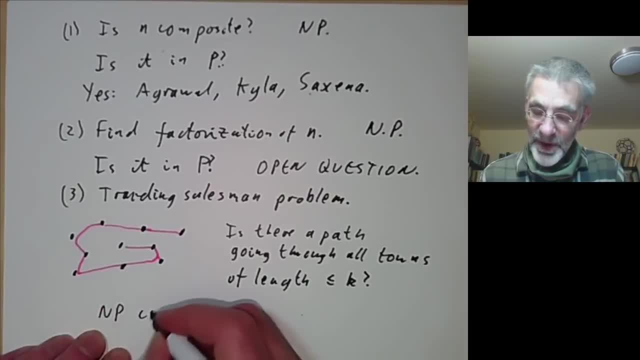 So this is an example of an NP-complete problem. If we could solve the travelling salesman problem in polynomial time, then we would be able to solve all other non-deterministic problems in polynomial time. So all you have to do to show that p is equal to NP. 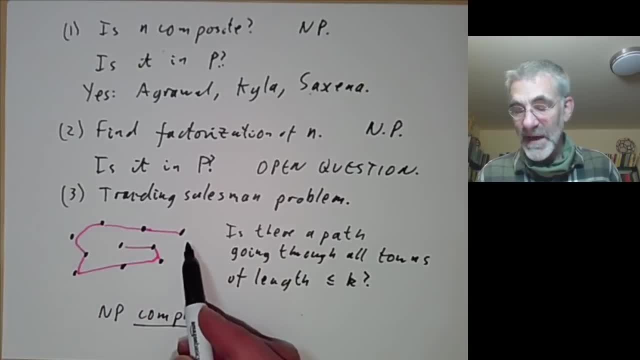 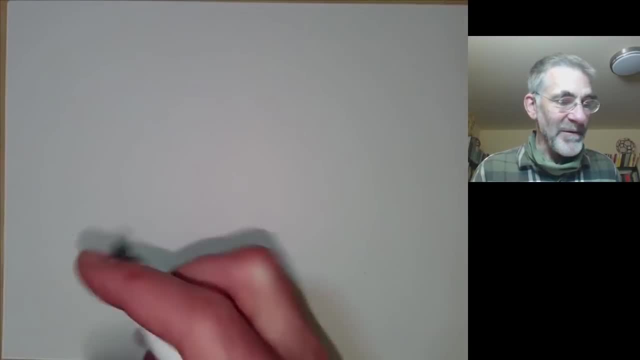 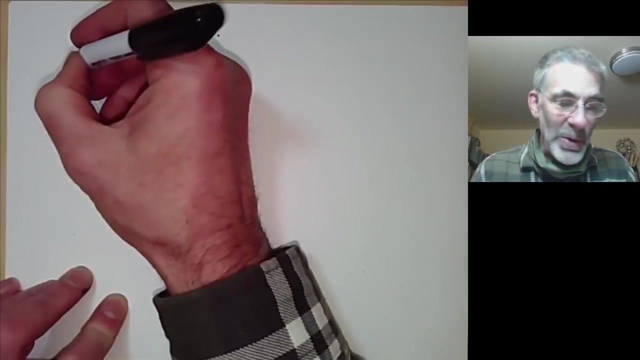 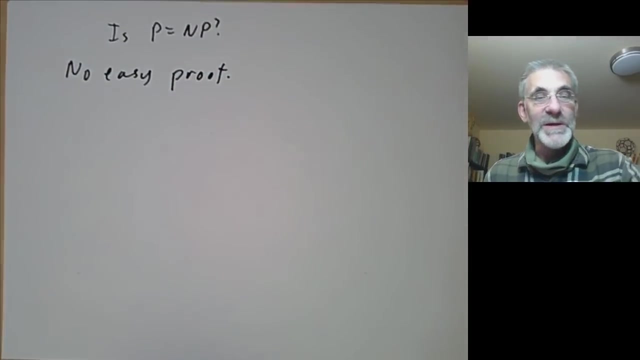 is to find an algorithm for solving the travelling salesman problem in polynomial time, And so far nobody has managed to do this. So we have the following question: Is p equal to NP? And there is no easy proof Either way. There's no easy proof and no easy disproof. 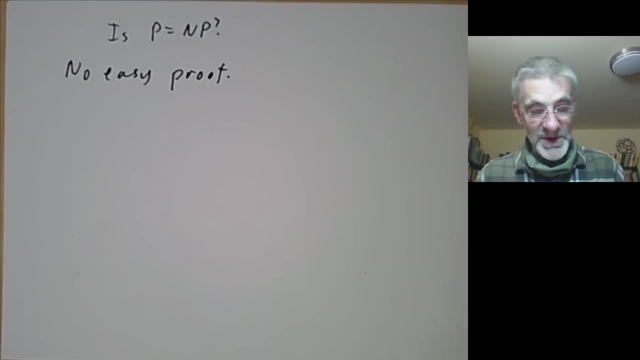 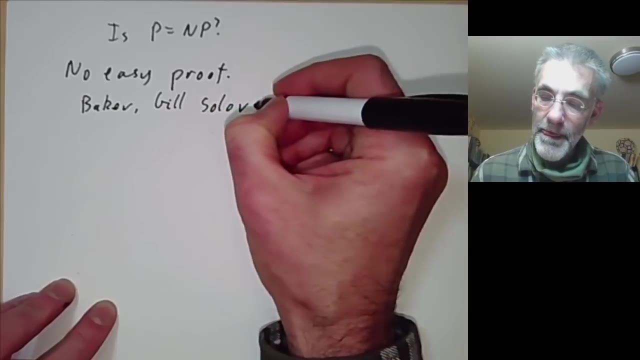 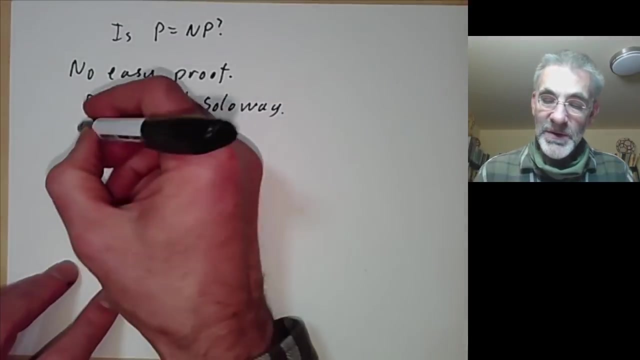 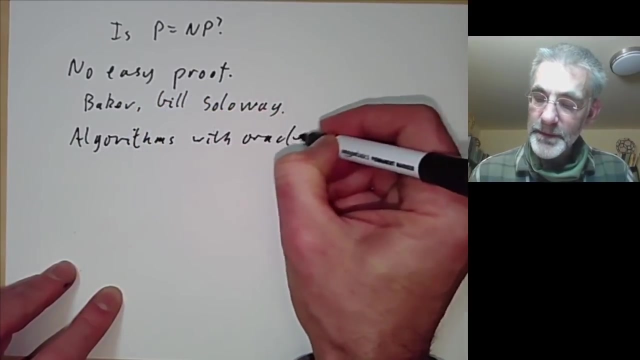 The first result suggesting that there was no easy way to do this was the result by Baker Gill and Solovey, And what they did was, instead of looking at algorithms, you look at algorithms with oracles. So an algorithm with an oracle means that your algorithm for doing something 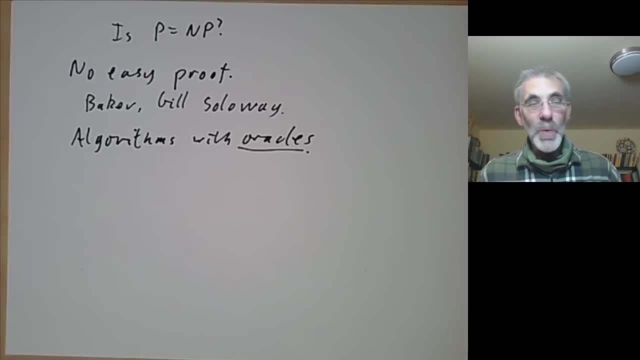 is allowed to stop every now and then and consult a wizard who knows the answer to a large collection of problems. So they will stop and ask the wizard some question and then take the wizard's answer into account and carry on. The wizard doesn't know the answer to absolutely every question. 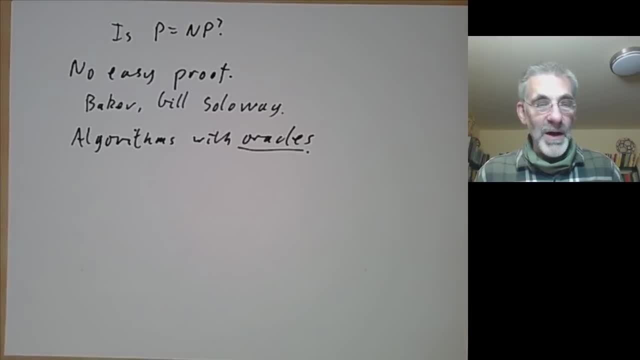 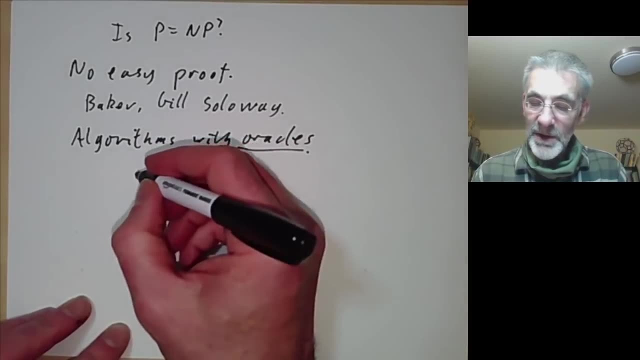 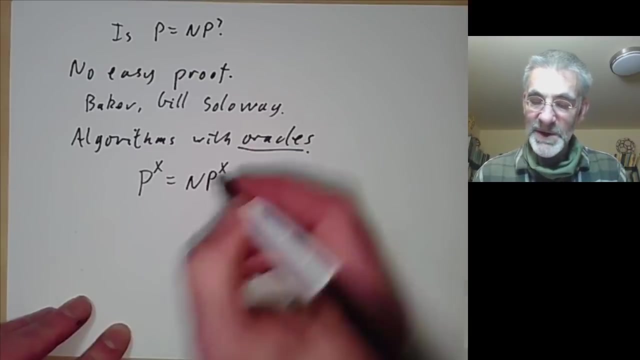 The wizard or oracle only knows the answer to a certain collection of problems. And what Baker Gill and Solovey did was they found a special sort of oracle, such that if you look at the polynomial time algorithms with oracle x, this is equal to the non-deterministic polynomial times with oracle x. 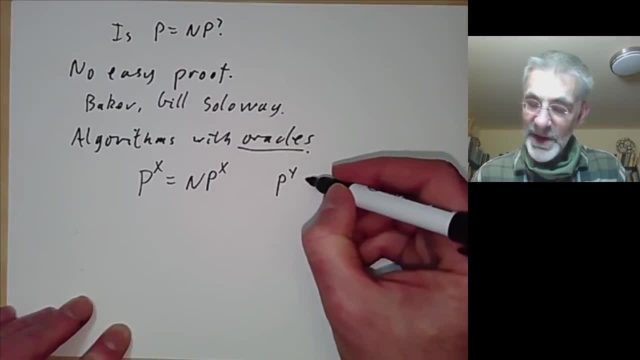 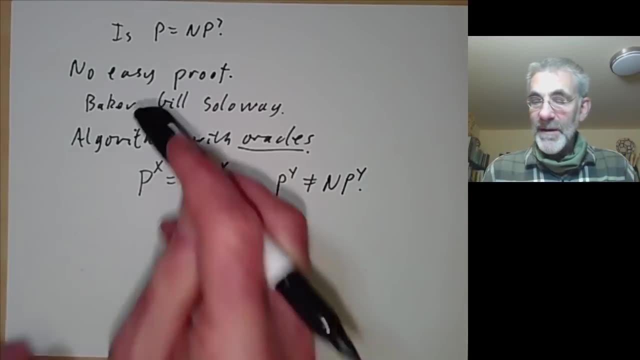 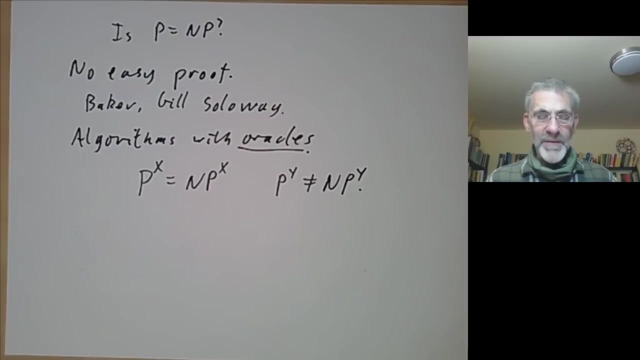 And similarly, they found an oracle y, such that p is not equal to NP. So if you allow algorithms to have an oracle, then this question can be either true or false, And this is a bit disturbing, The reason being that most of the methods we know for proving theorems 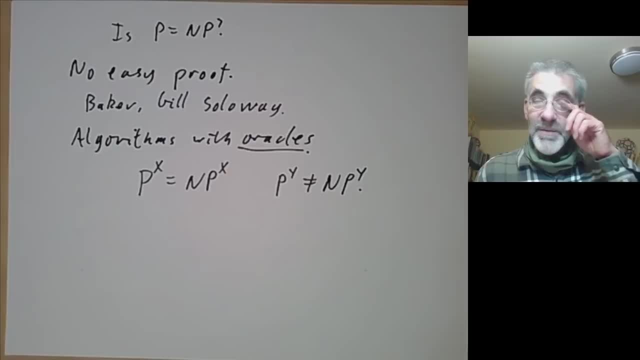 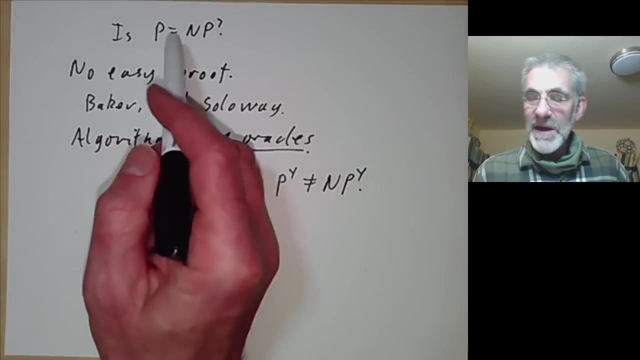 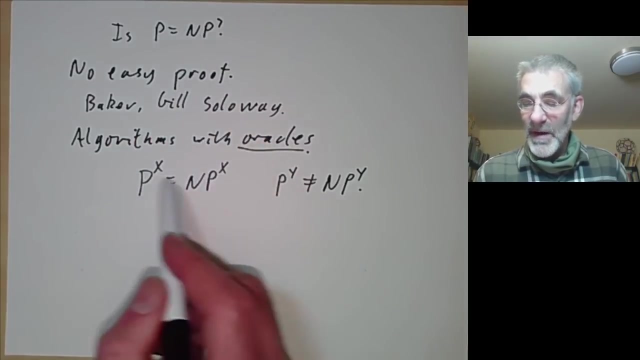 about speed of algorithms go through with very little change to algorithms with oracles. This means that if there was any proof, using easy techniques, of this question here, then it would also apply to algorithms with oracles, but that actually depends on which oracle you're looking at. 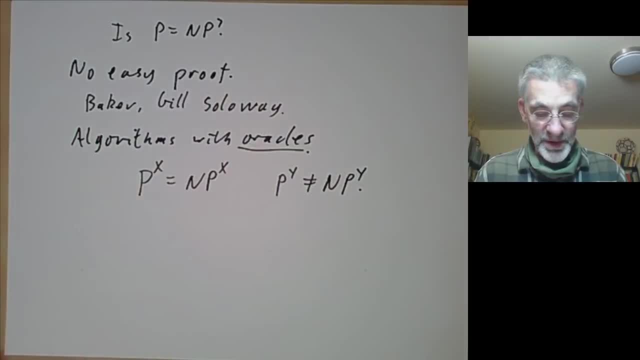 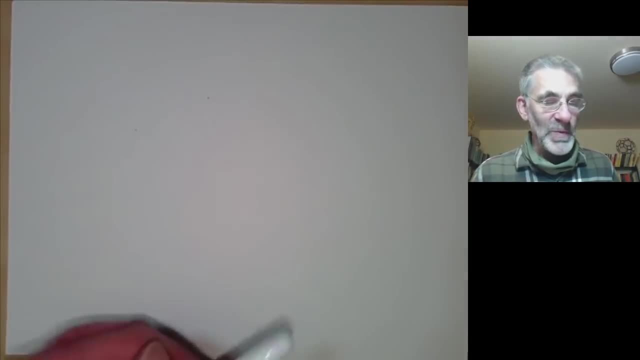 So the proof can't work for all oracles. So now I want to say a bit about whether Let's look at the evidence for or against the question of whether p is equal to NP. So the first thing you do if you've got an unknown question. 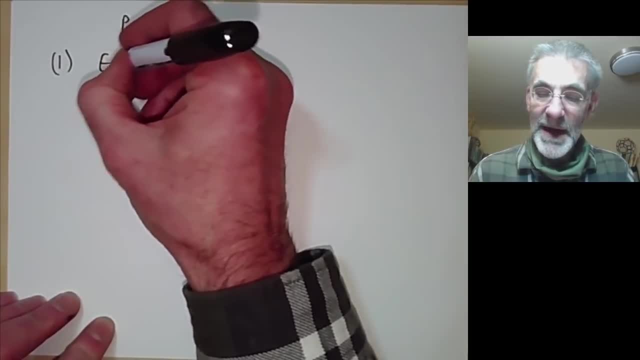 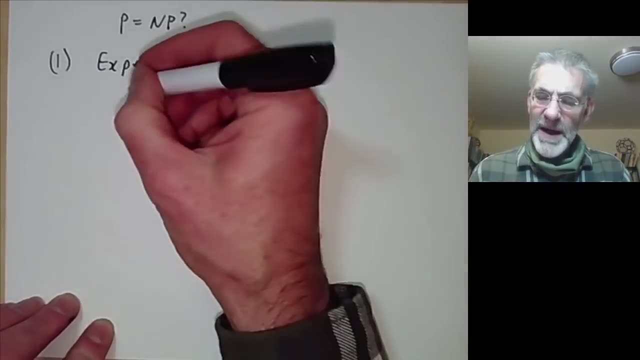 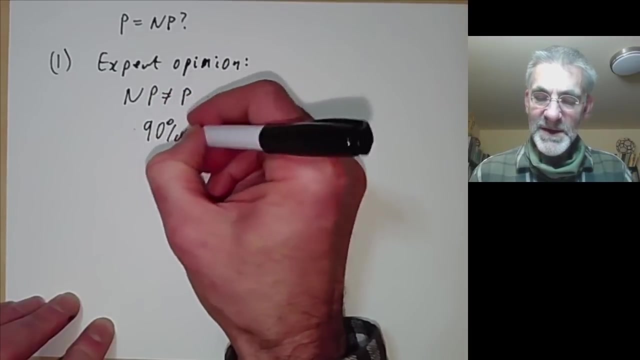 a question. a subject you don't know much about is to ask about expert opinion. So let's consult this. Well, the expert opinion for p not equal to NP- about People have done surveys and something like 90% of people working on it. 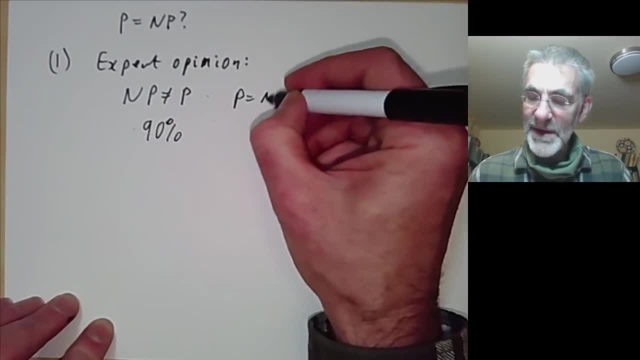 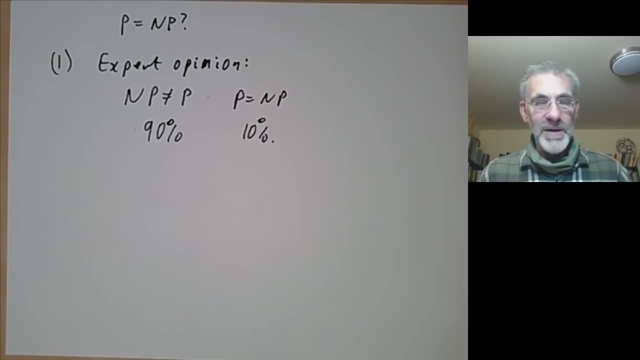 think the answer is that they're not equal. And for p equals NP, about 10% think the answer is yes. Well, you've always got to be a little bit careful about expert opinion, You know, if you wanted to know about some result in, say, parapsychology. 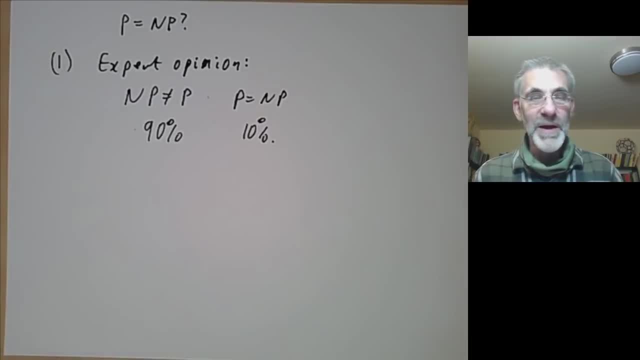 or astrology or something, and asked for expert opinion. it might not be terribly reliable. The trouble is that any expert on parapsychology has probably chosen to work in parapsychology, which means they probably haven't yet figured out that parapsychology is complete bunk. 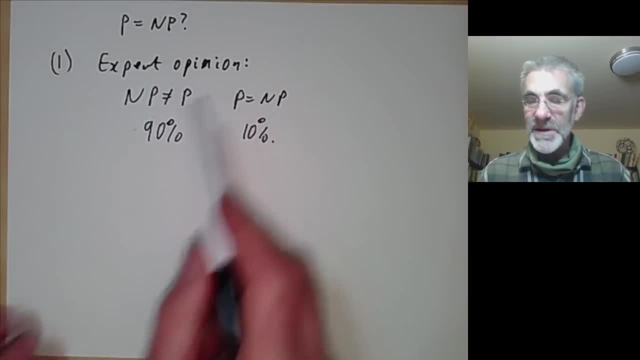 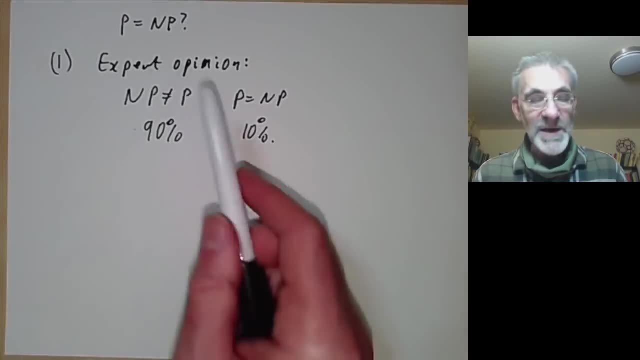 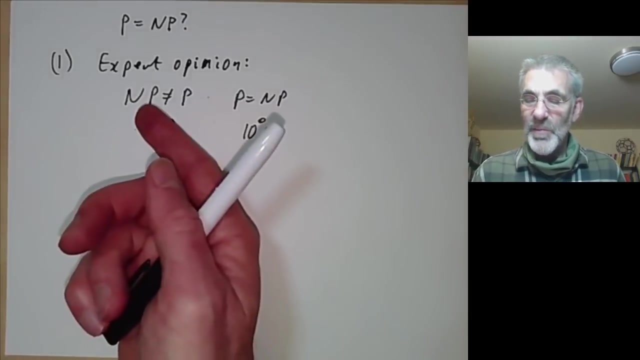 So expert opinion is fine, as long as your subject is non-flaky, Well, that's okay, because computer science and computation is definitely a non-flaky subject. So expert opinion in this case is probably reasonably reliable, And the default assumption seems to be that p 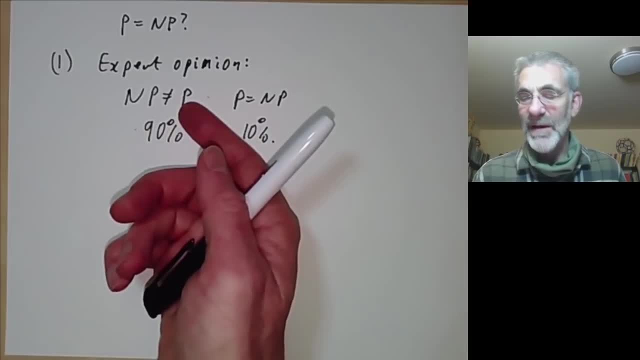 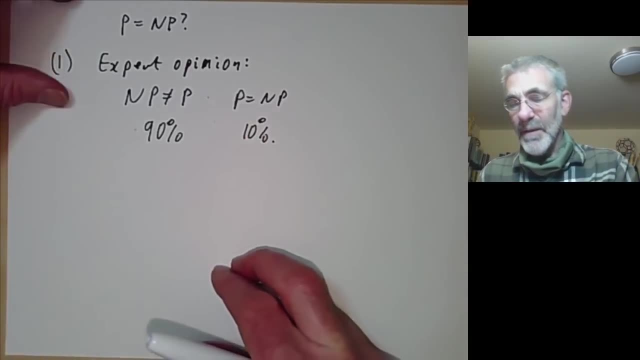 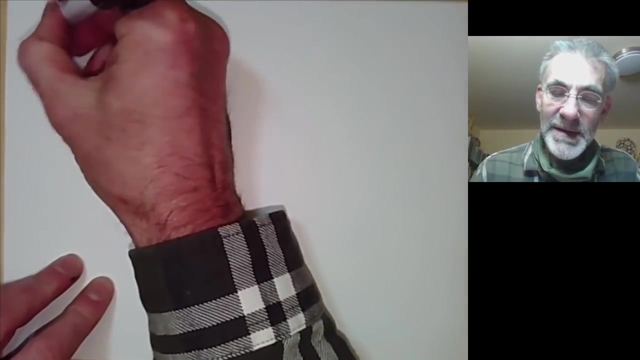 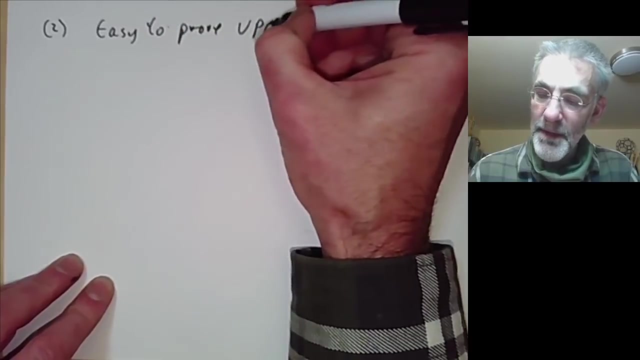 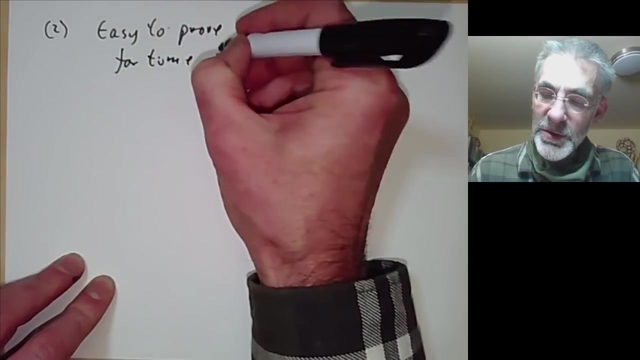 We should sort of expect that p is not equal to NP, but there's a certain amount of reasonable doubt about it. So now let's For another argument. let's observe that it's easy to prove upper bounds For the time to solve something. 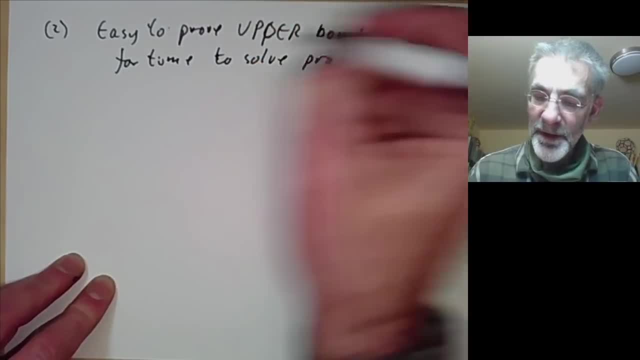 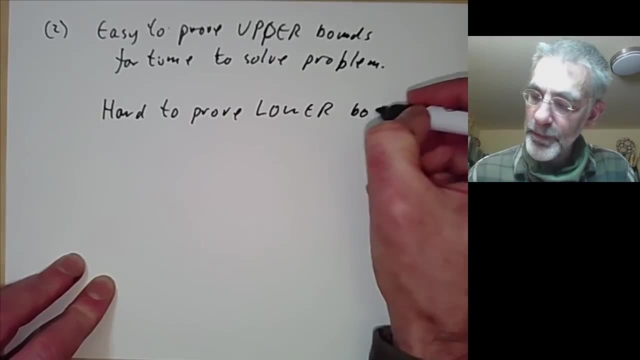 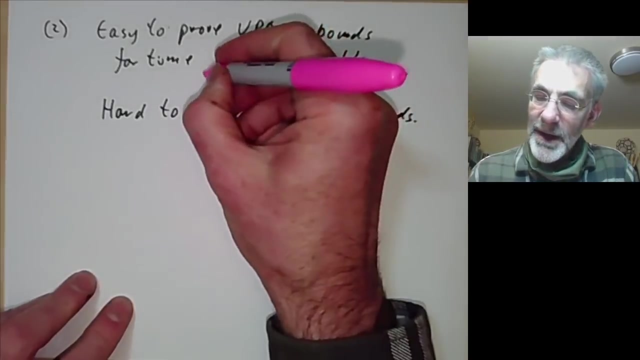 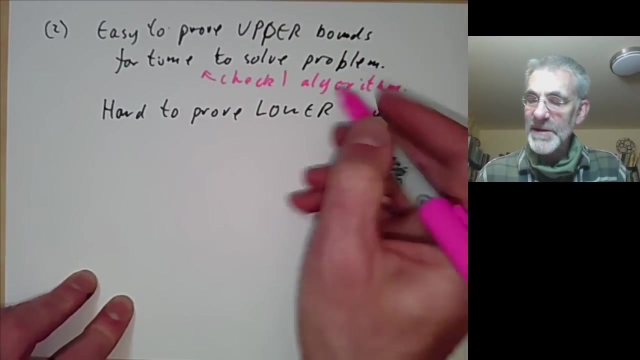 On the other hand, it's hard to prove lower bounds, And the reason for this is very simple: If we want to prove an upper bound, all we have to do is to check one algorithm, And we just have to show that this one algorithm is fast. 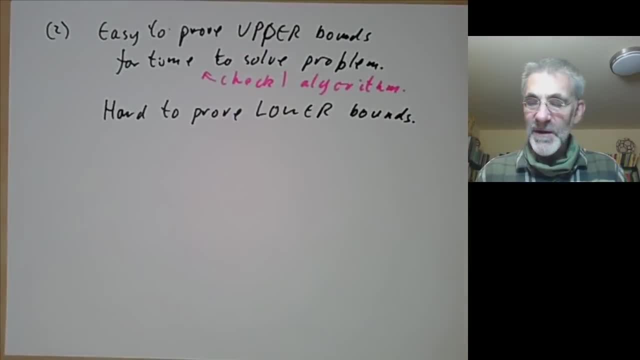 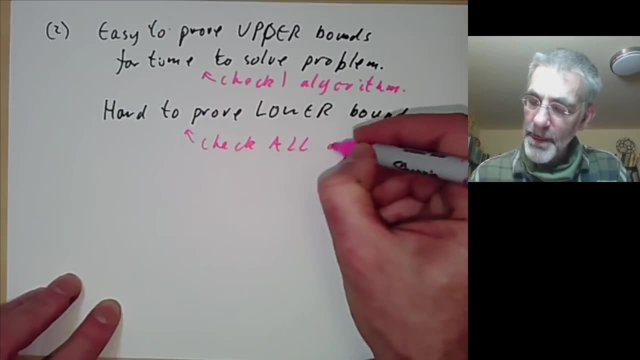 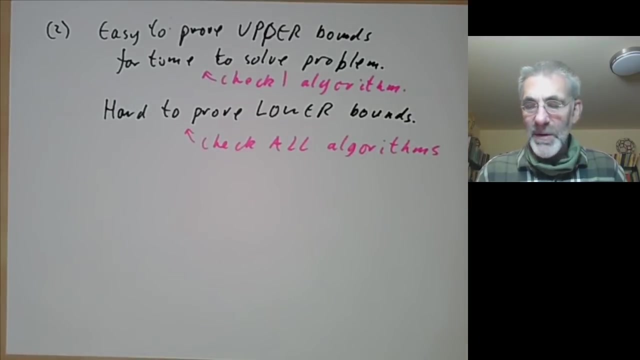 and that gives us an upper bound for the time taken to solve a problem. However, if we want to prove a lower bound, we need to check all algorithms. Of course, we don't need to check them individually, one by one, but we somehow need some argument that will check all algorithms. 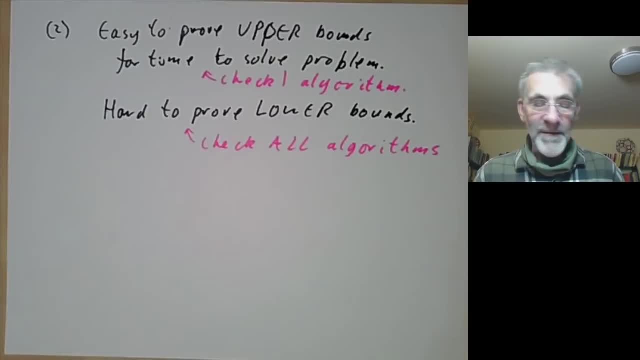 because we've got to check that every single algorithm doesn't somehow cleverly solve our problem. So, um, So, upper bounds. So upper bounds, you only have to check one thing, but lower bounds, you have to check an infinite number of things. 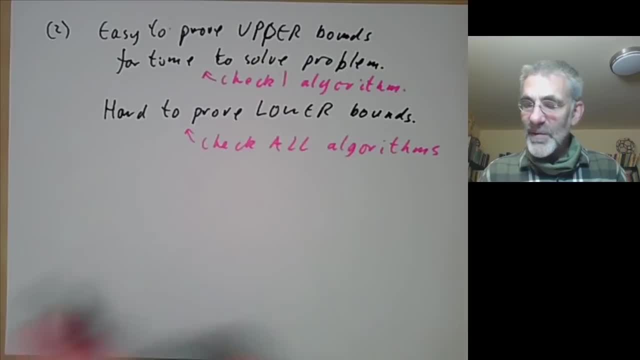 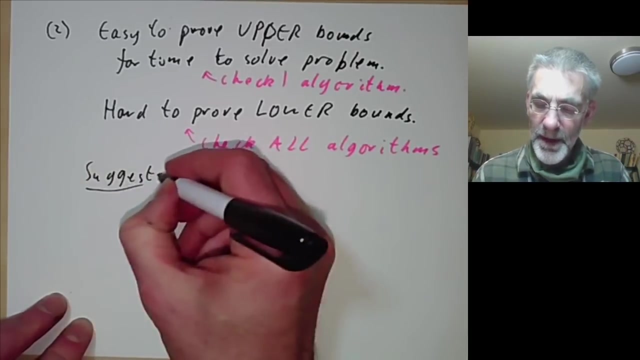 so it's much harder to do this. This means if we are unable to decide how fast the best algorithm is, it's more likely to be quite slow, because it's the lower bound. that's hard to prove. So this suggests P is not equal to NP. 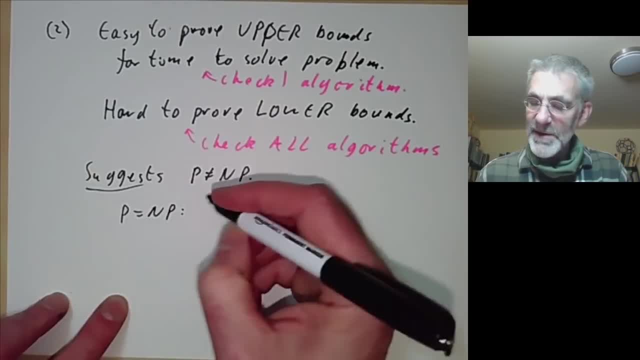 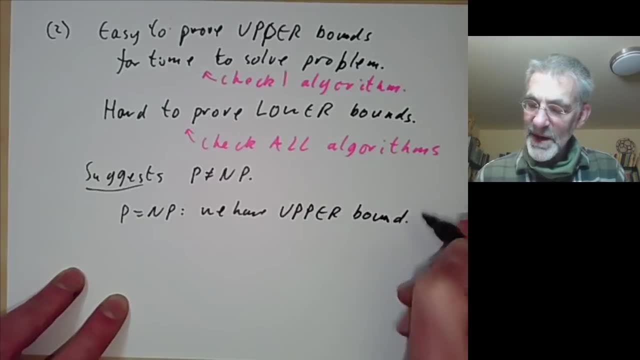 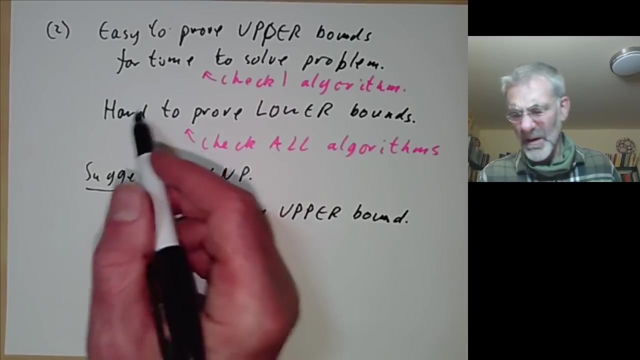 Because if P was equal to NP, this would mean we have an upper bound. Showing P equals NP means we need to find a polynomial upper bound for an NP-complete problem, and we haven't managed to do that. which sort of hints that maybe there isn't one. 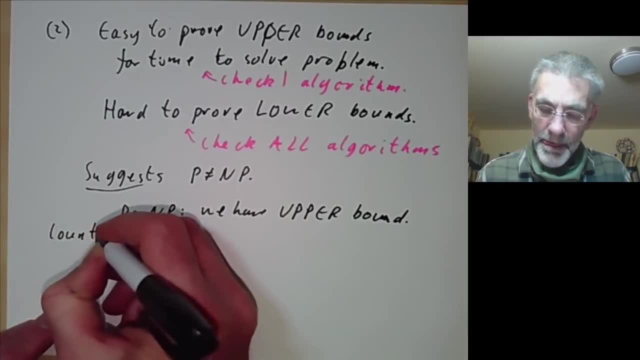 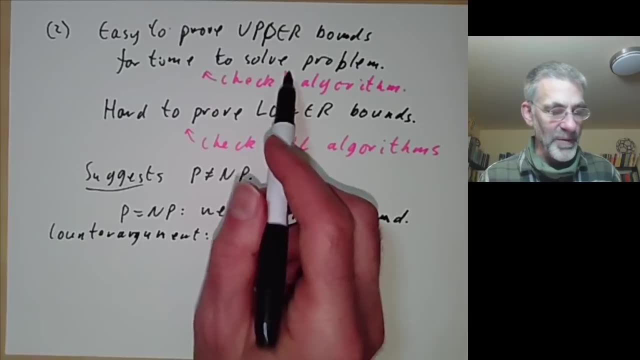 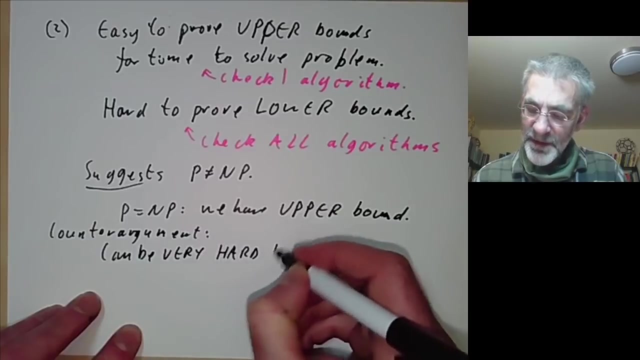 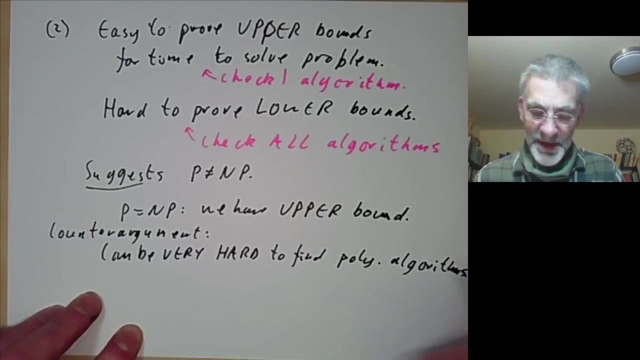 Well, let's have a counter-argument. Well, the counter-argument is that it's not always easy to prove polynomial upper bounds, So it can be very hard to find polynomial algorithms. So let's have an example of this: Um. 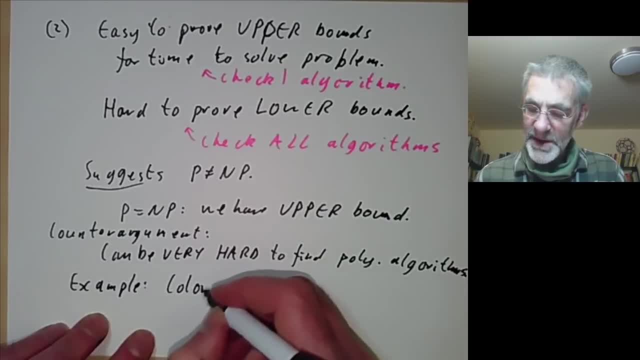 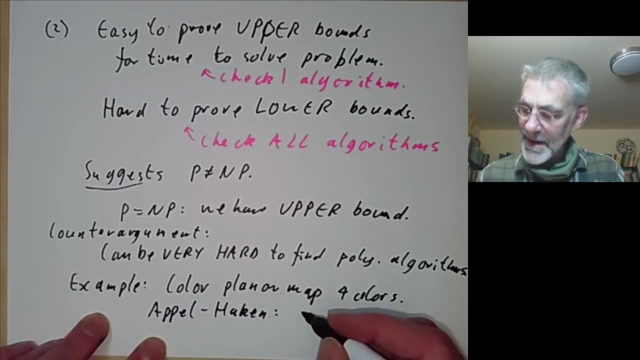 Suppose you take a planar map and you want to colour it with four colours. Now Apple and Harkin showed that there is a polynomial time algorithm for doing this. The trouble is, it's incredibly difficult to prove that there is a polynomial time algorithm for doing this. 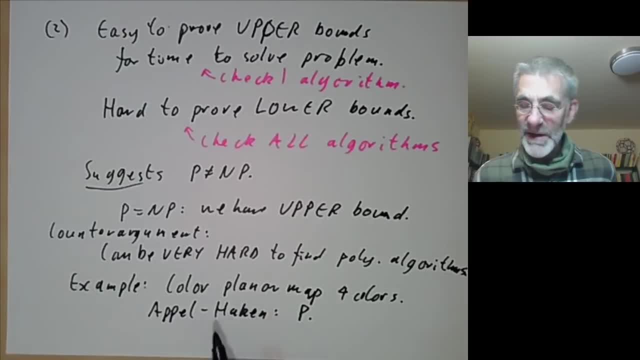 In fact, as far as I know, no human has ever actually read a proof of this. OK, so how do you prove it if no human has read a proof? Well, the answer is: a lot of the proof was done by computer calculation. 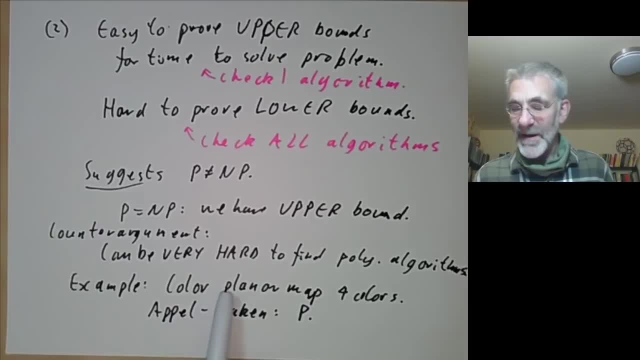 You have to check enormous numbers of complex numbers and you have to do a lot of complicated cases to show that the algorithm they gave actually works. So it can be. You know there may be polynomial time algorithms that are really difficult to find and prove. 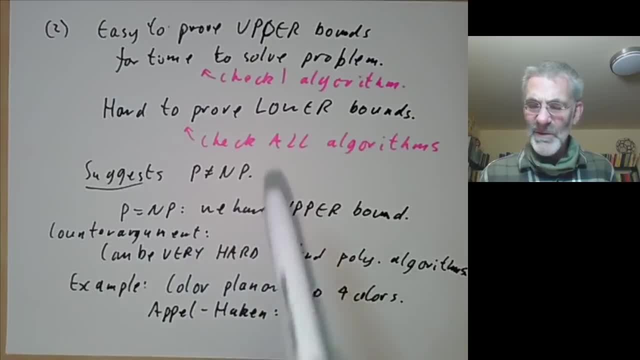 So the conclusion of this is that algorithms are really very poorly understood. So, although this suggests that p is not equal to np, what it's really doing is it suggests that either p is not equal to np or that we're kind of stupid and don't really understand algorithms. 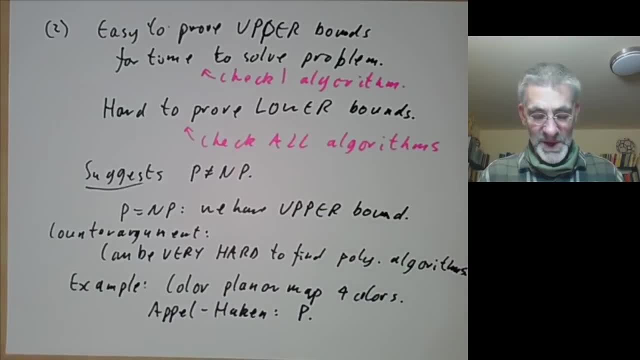 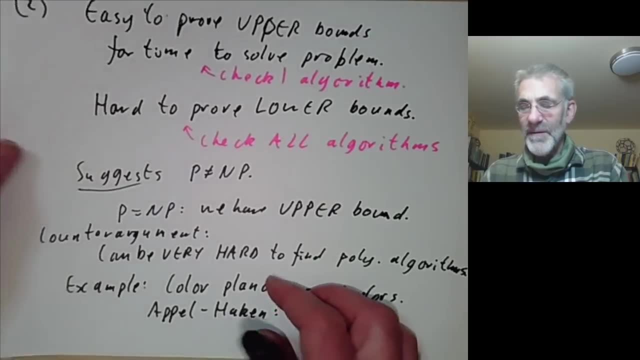 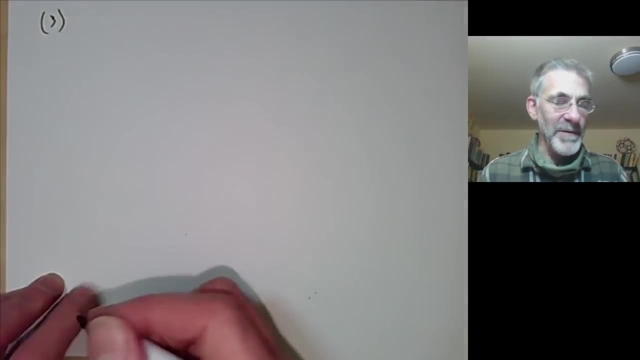 And as we're kind of stupid and don't understand algorithms, it doesn't really give a whole lot of information. So there's some very weak evidence in favour of the fact that p is not equal to np. Now I'll come on to something that I think is somewhat stronger evidence. 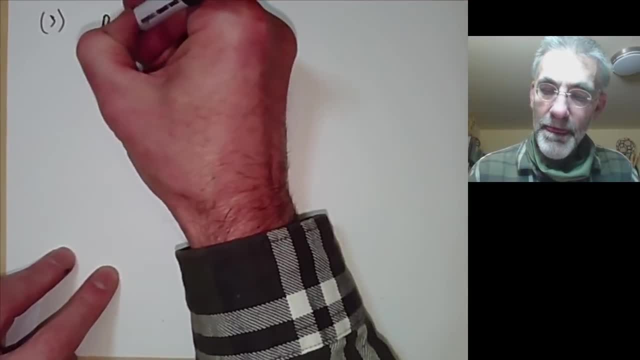 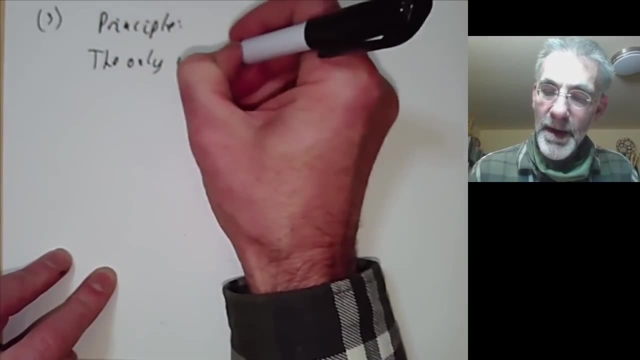 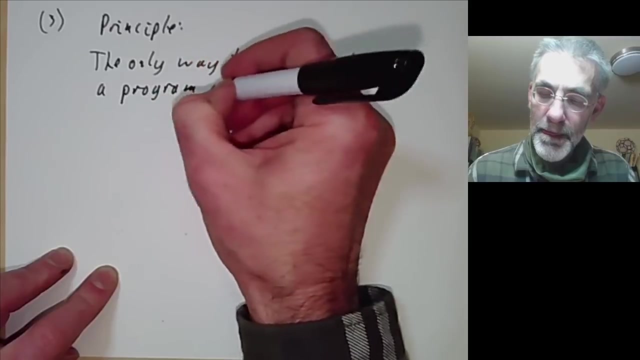 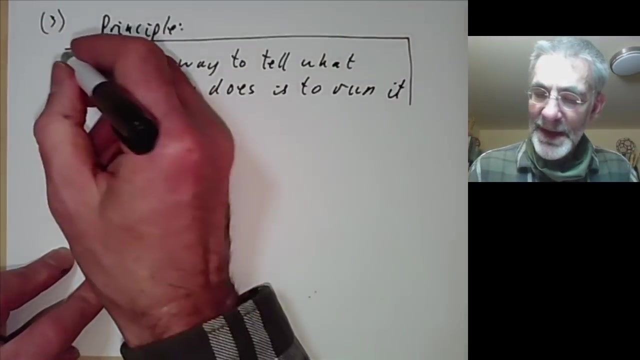 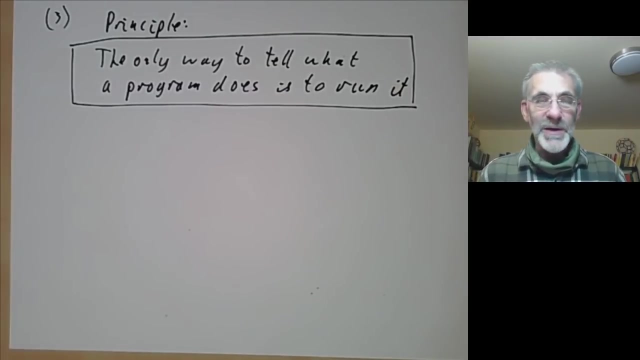 This depends on the following principle, a slightly informal principle, which says the only way to tell what a program does is to run it. Well, that's for general programs. I mean, most of the programs you actually come across are specially written to make them easy to understand. 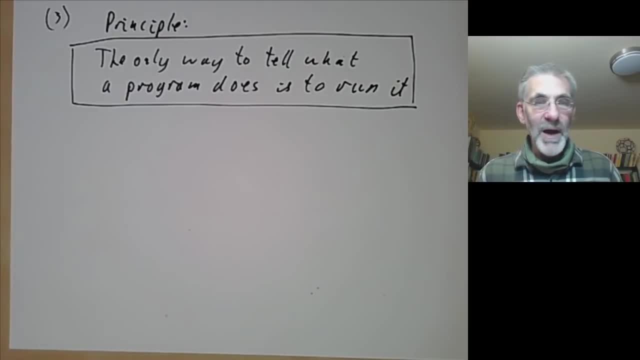 I mean they have to be documented and written in a simple way, and so on. But these are very untypical of most algorithms. Most algorithms are almost impossible to understand. If you've ever tried to read someone's poorly written, undocumented code. 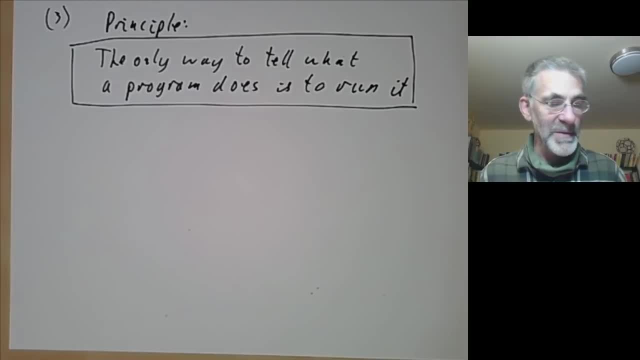 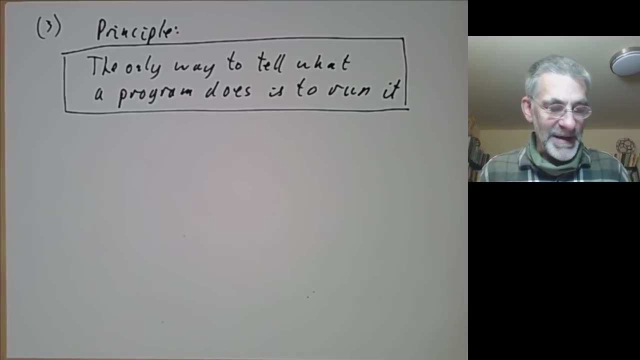 you will know what I mean. It can be really hard to figure out what code is supposed to be doing. In fact, there's a competition called the Obfuscated C Contest, where people deliberately try and write code in C that's as difficult to read as possible. 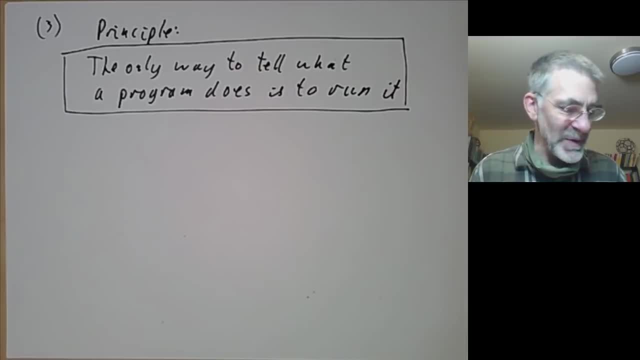 I don't really know why, because code in C is always a bit difficult to read, even if you're not trying to obfuscate it, And there are some really impressive examples. For instance, here is an example written, I think, by Brian Westley. 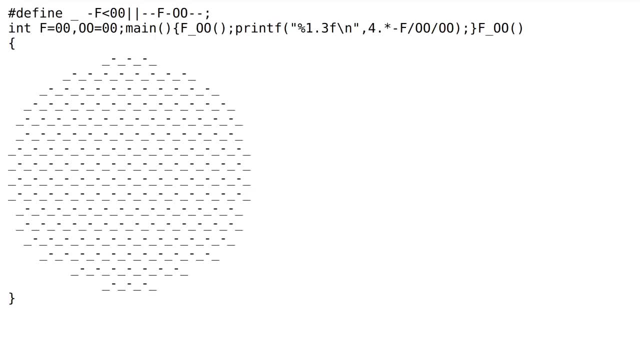 And so I have a problem for you. What does this program do? And even if you are an expert, experienced C programmer, if you look at this, you probably haven't got the faintest idea what the program does, And it would take you several hours to figure out what it does. 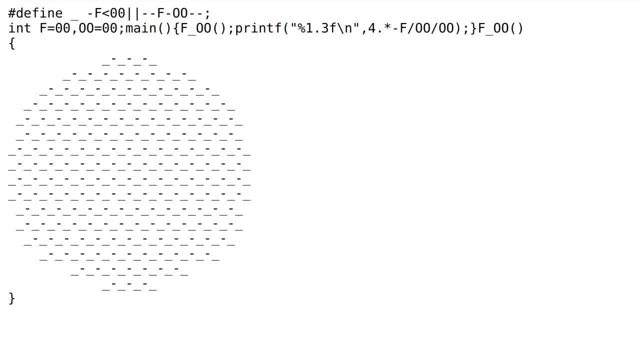 even though the main part of it seems to be only two lines long and seems to be little more than a couple of definitions, What it actually does is it calculates pi by calculating its own area and then dividing that by its own diameter. You see that the program sort of looks a bit like a circle. 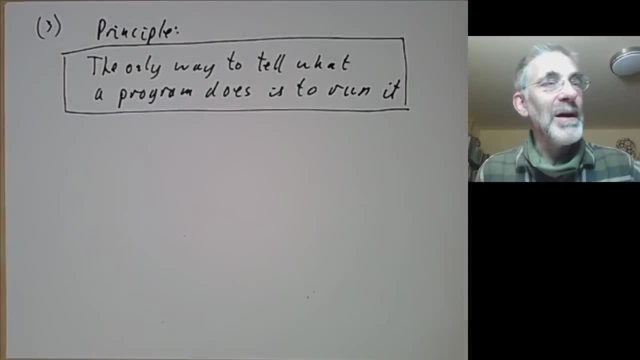 So that's just an example to show how difficult it can be to figure out what a program does. Incidentally, that's one of the easiest programs in the obfuscated C competition to understand If you go and look at some of the others. 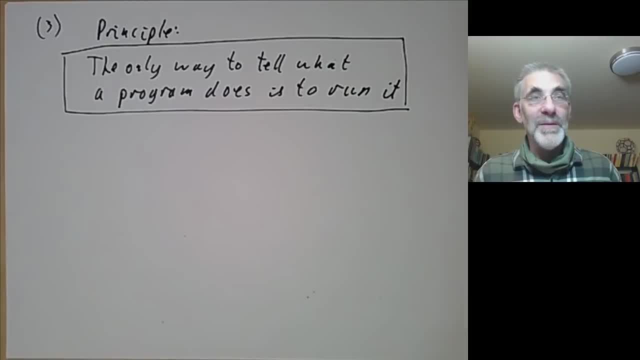 they are absolutely bizarre. I mean, you sort of look at them and there's just no way you can figure out what on earth is going on there. There's an extraordinary amount of ingenuity and time-wasting gone into this competition. So the point is that, examining the code for a program, 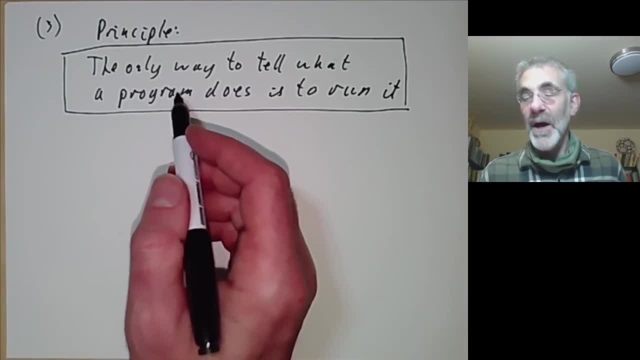 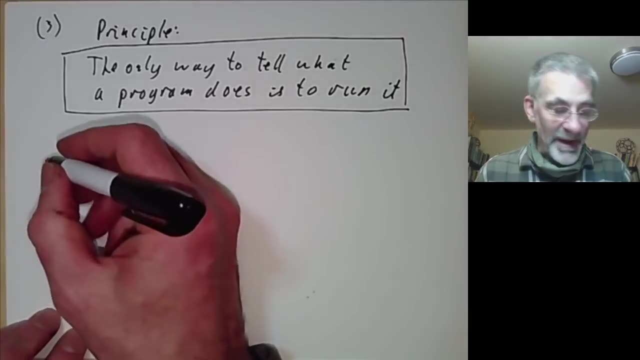 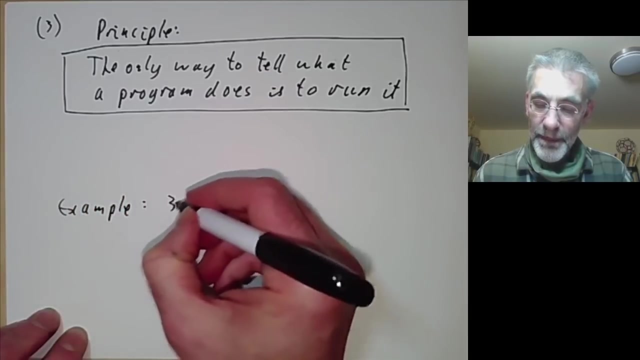 or an algorithm in general, gives no useful information beyond what you can find by simulating the program or running it. Another example of this is the 3x plus 1 problem. So this is a rather famous problem. It says: you take an integer x. 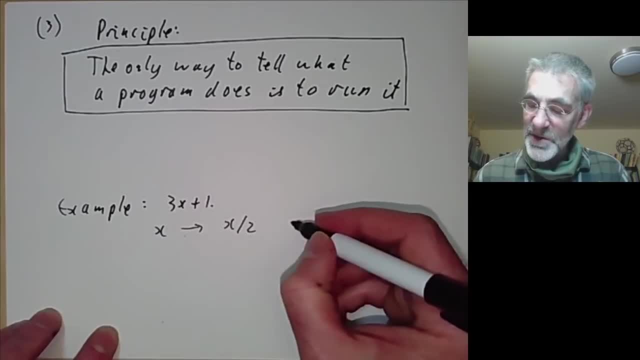 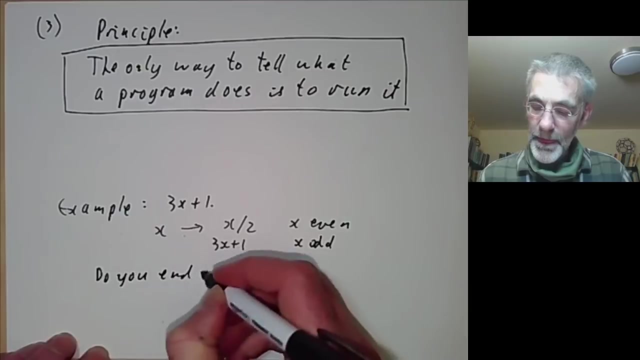 and if it's even, you map it to x over 2, and if it's odd, you map it to 3x plus 1.. And you keep iterating this and you can ask: do you end up at 1 for all integers? 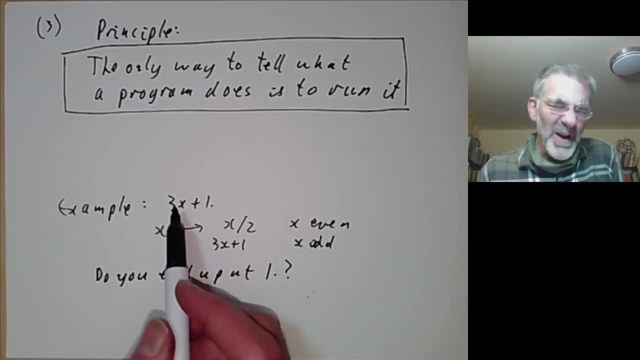 So this is a very simple program. It's hard to think of anything simpler than doing this to an integer, And you just ask. you know, if you iterate that often enough, do you always end up at 1? And nobody knows. 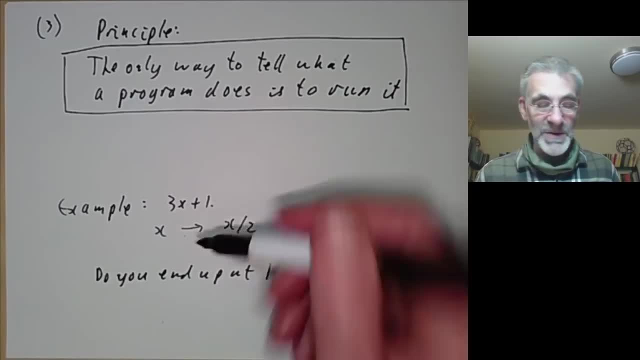 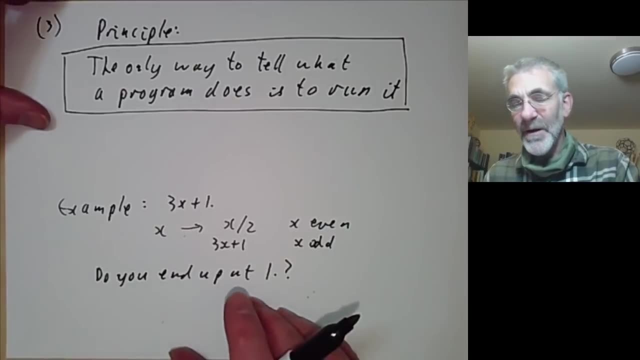 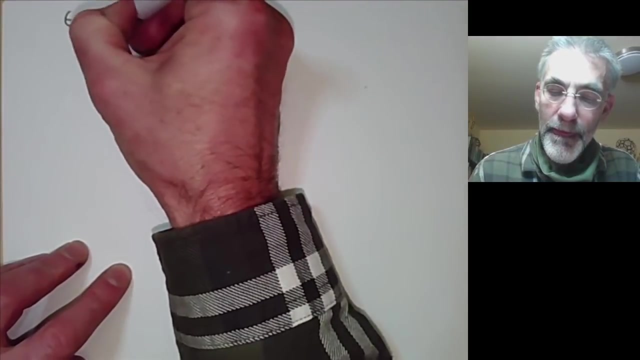 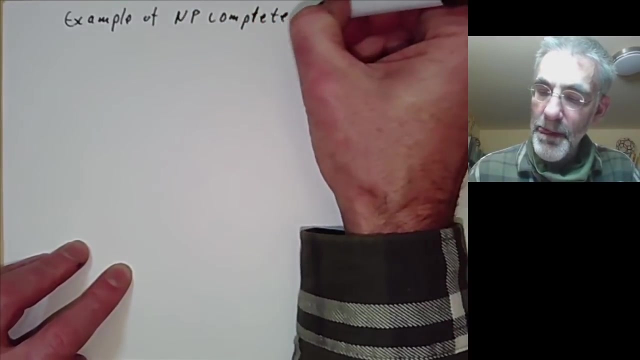 This program is incredibly difficult to understand its behavior. So even for very simple, clear programs like that, it can be very hard to understand what they're doing. So let's have an example of an NP-complete problem. Well, I gave an example earlier. 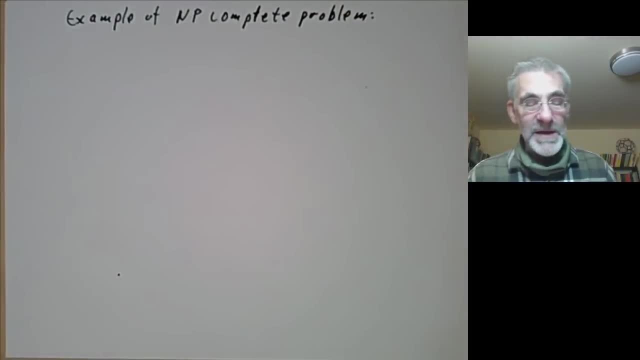 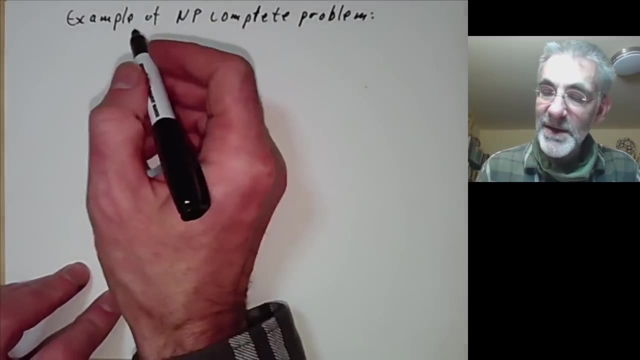 of the traveling salesman problem, but it's a little bit difficult to see that it's NP-complete. It's obviously NP but completeness is a bit difficult. So here's a problem that's almost obviously NP-complete. So it's going to take as input. 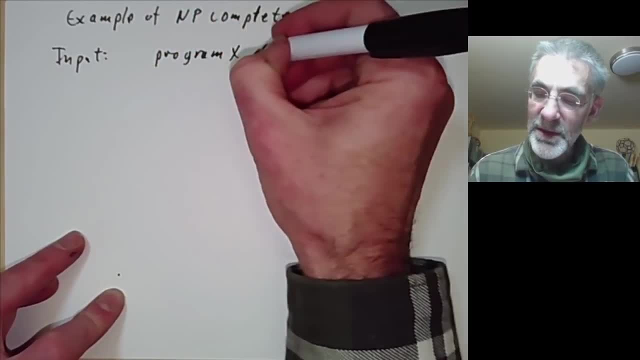 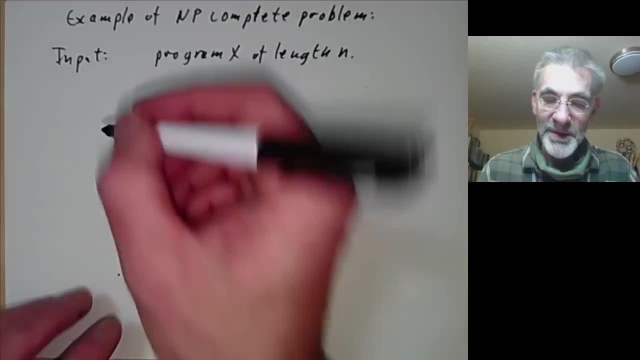 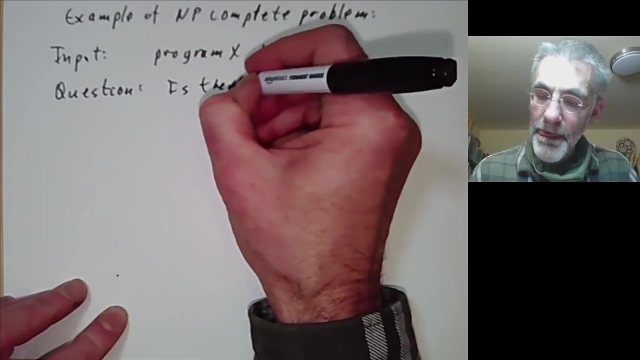 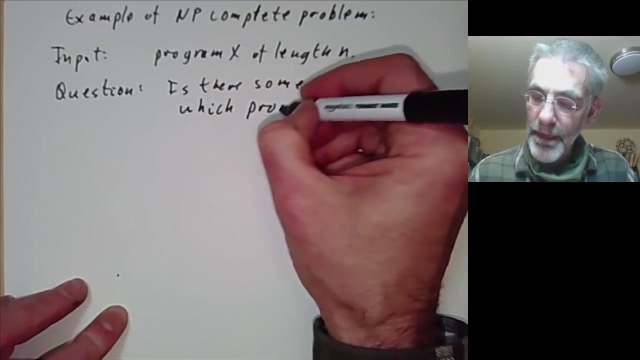 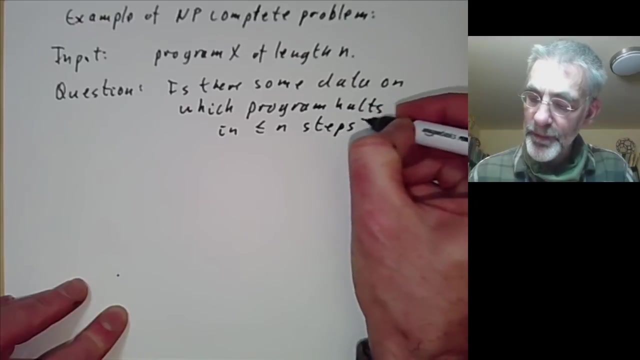 a program x of length n written out in. you know it could be a Turing machine of length n or something And you have to answer the following question: Is there some data on which the program halts in less than or equal to n steps? 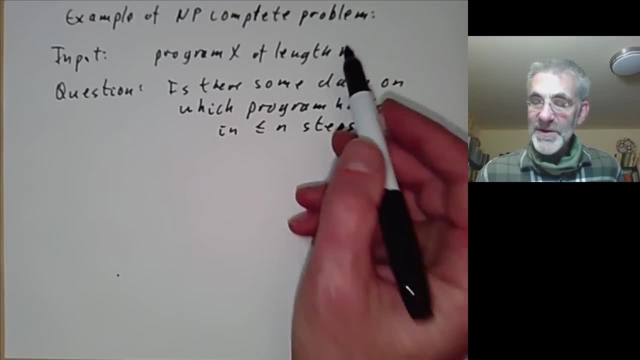 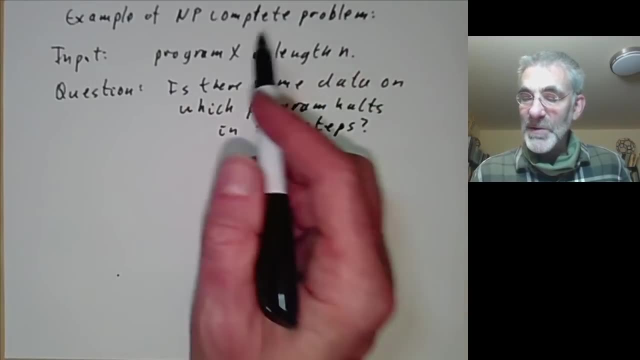 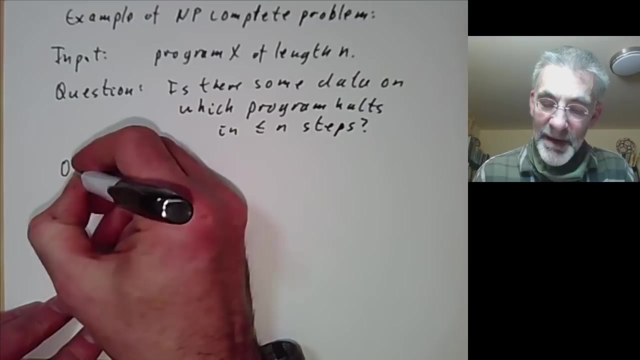 So you fix a number, n, and you want to have an algorithm that takes most polynomial time in n, which will tell you, for any program of length n, whether there's some data on which it halts. And this is obviously NP, because if we're given a program, 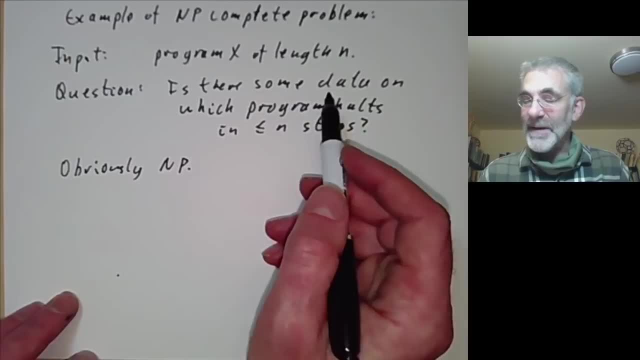 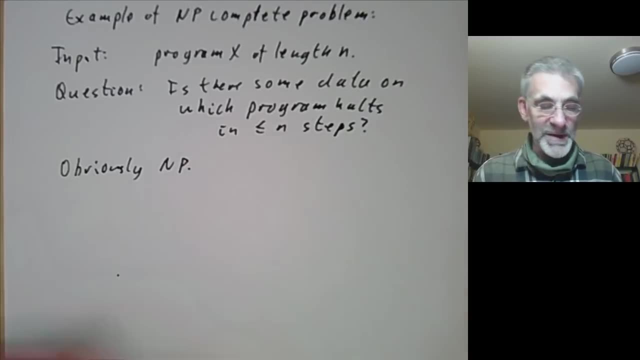 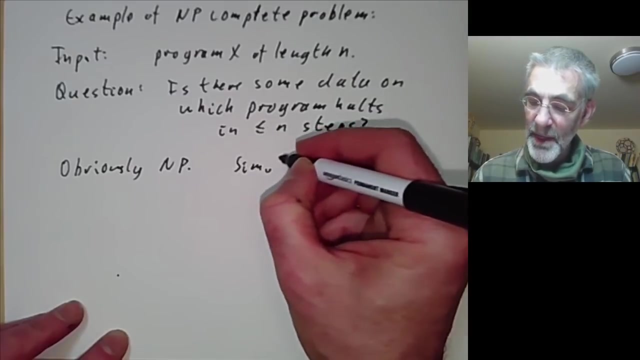 and it halts on some data of length n. then we can just write down this data by, you know, randomly guessing it, and check by simulating the program that it halts in most n steps. So it's obviously NP. We just simulate our program. 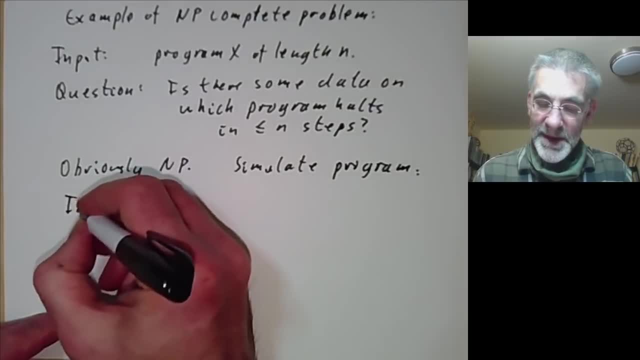 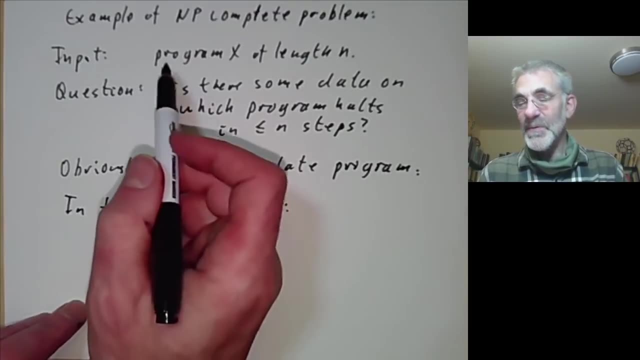 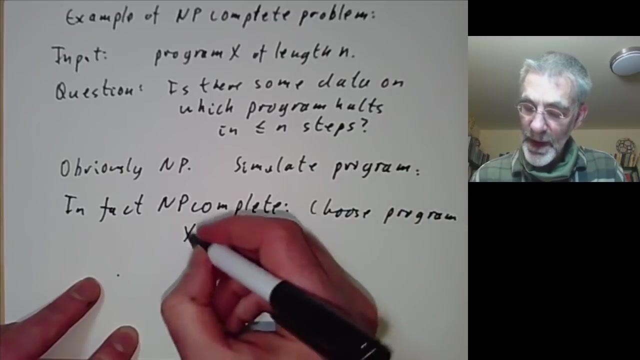 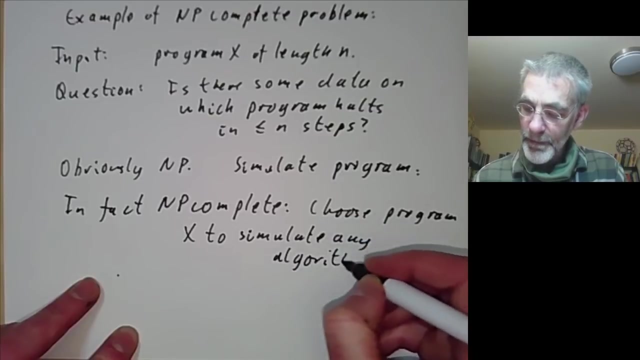 It's a little bit more difficult to check that it's NP complete And the point is that since we're allowed an arbitrary program here, we can just choose the program x to simulate any algorithm. And from this, if you can answer this question, 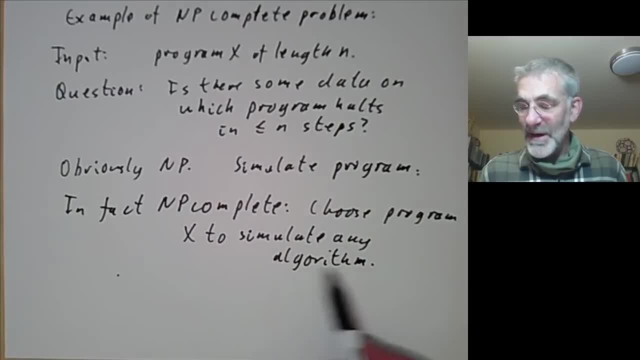 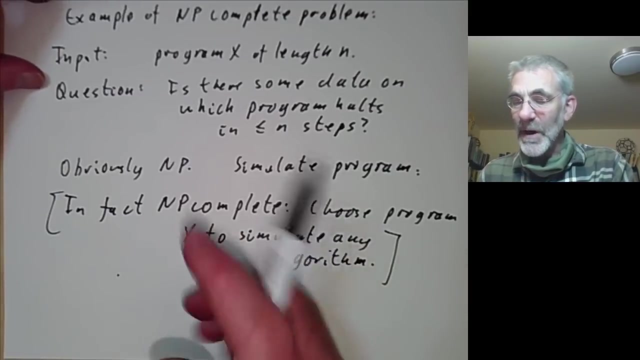 in polynomial time, then by using x to simulate any algorithm, you can basically check whether any algorithm halts on some input in polynomial time. So in some sense this problem here is the archetypal example of an NP complete problem. Well, suppose we try and answer this question. 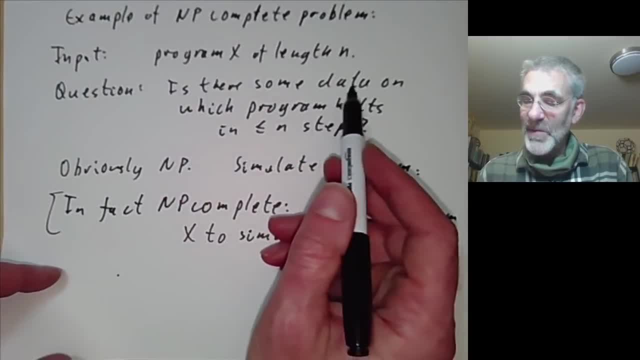 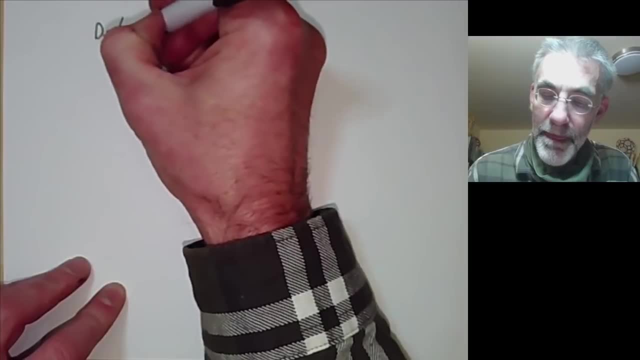 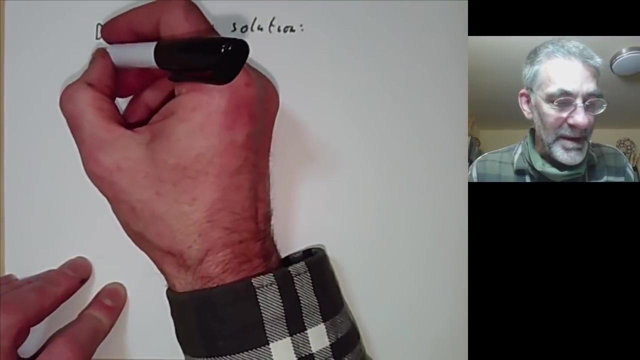 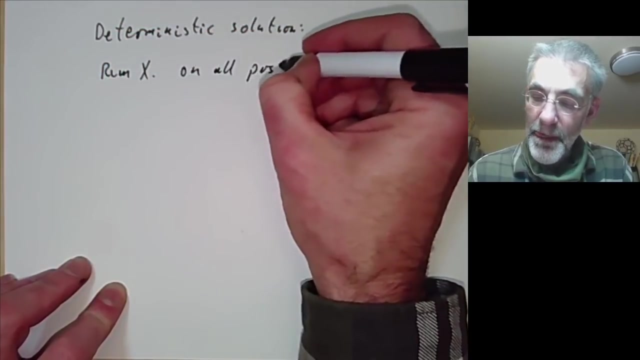 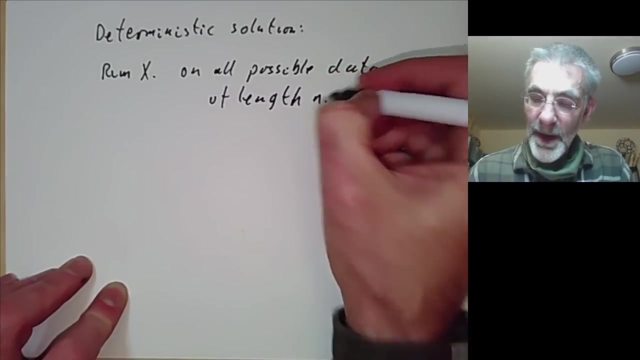 deterministically. So we can see whether there's some data on which the program halts by guessing the data. So here's a deterministic solution. What we do is we run x on all possible data of length n And we check for each of these. 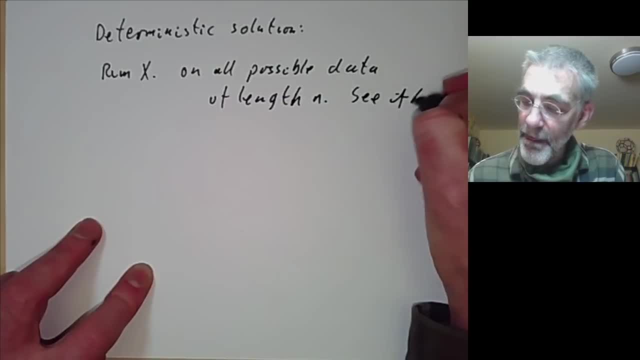 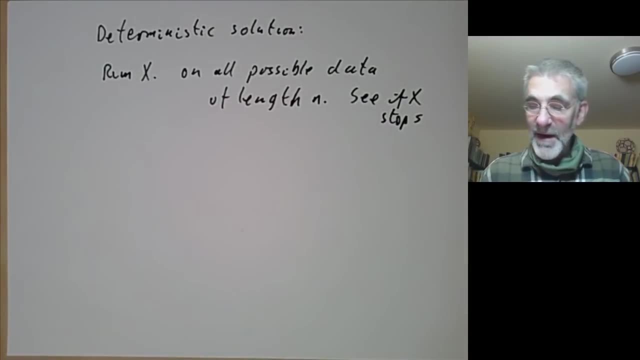 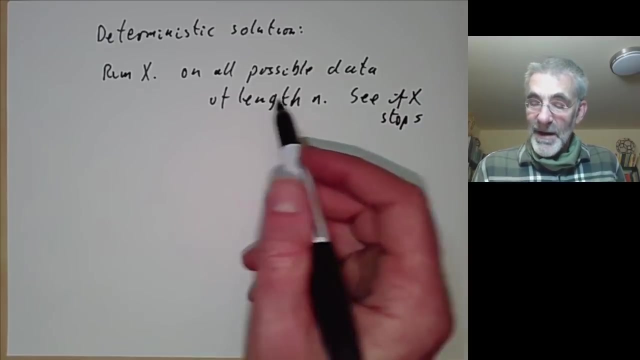 to see if x stops. So we can certainly check to see if there's some data on which x stops at length at most n deterministically. And you notice we only have to run it on data of length n, because if we're running the program 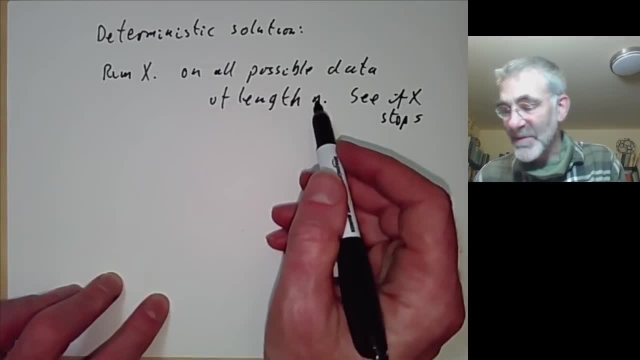 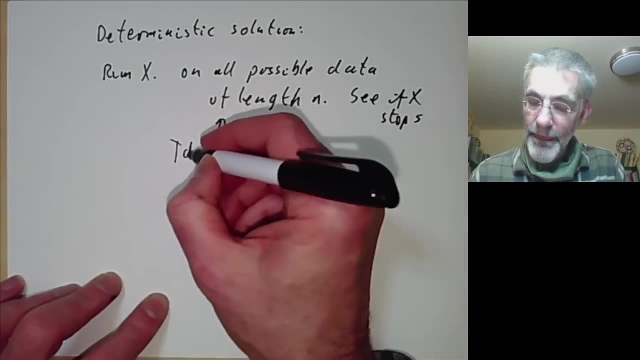 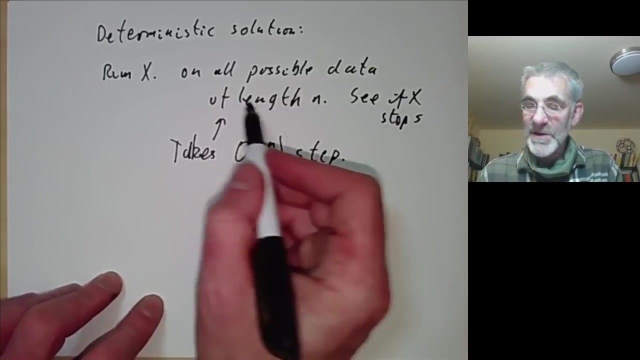 we want to check to see if it stops at most n steps. So it can't read more than n data points. And how long does this take? Well, it takes about 2 to the n steps, because there are 2 to the n possible choices. 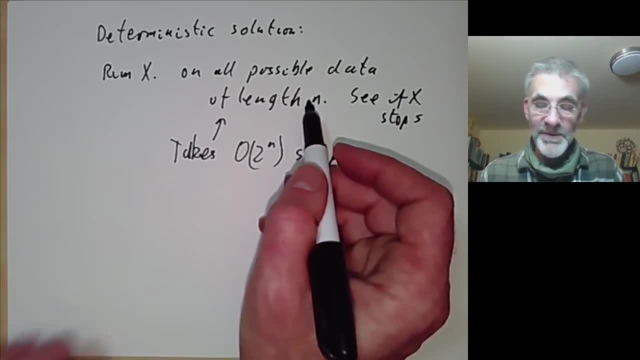 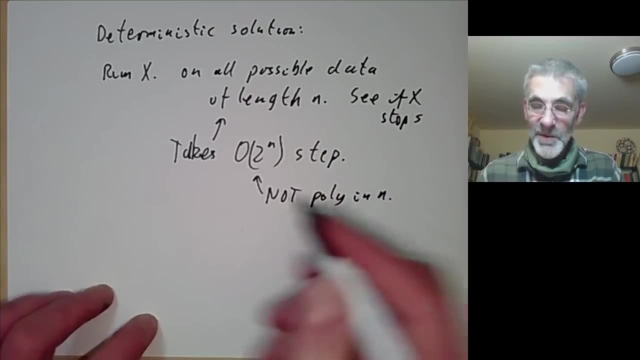 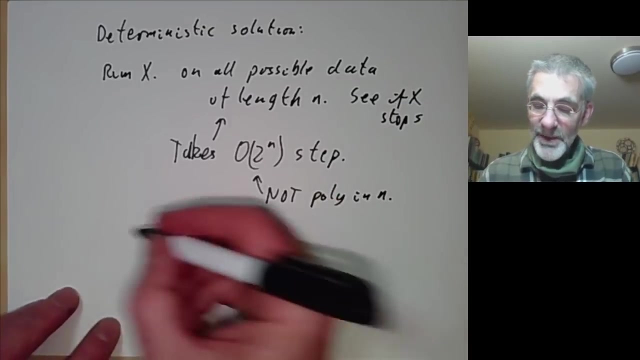 for the initial data of length n, assuming the data is in binary or something, And we notice the problem: This is not polynomial in n. So the obvious way of solving this problem doesn't run in polynomial, It runs in polynomial time. Well, what can we do in polynomial time? 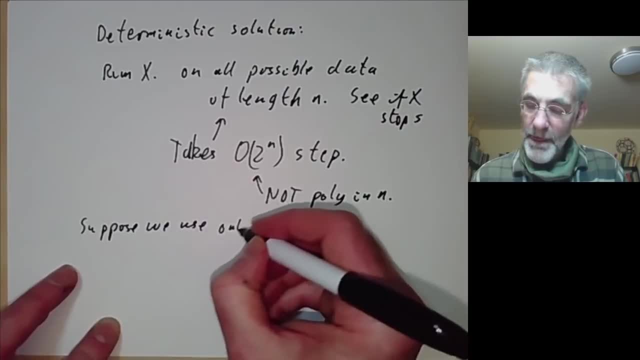 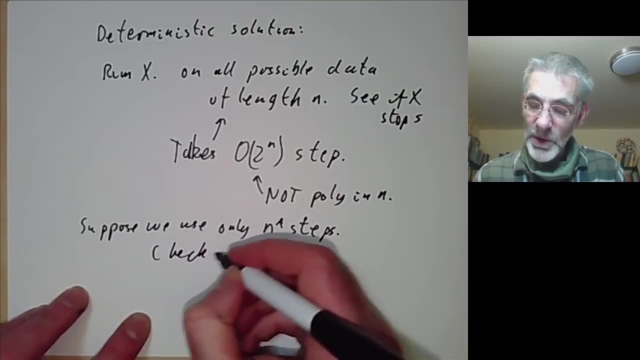 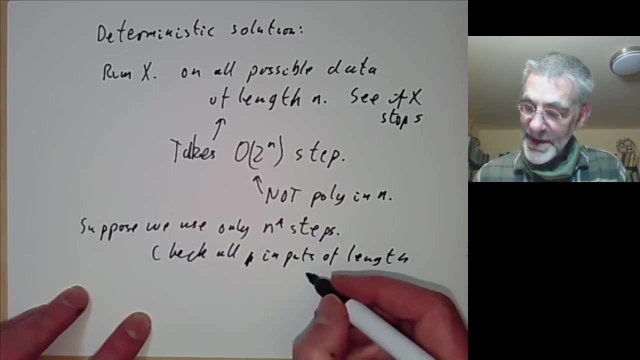 Suppose we use only n to the a steps, which is some polynomial, Then we can check all inputs of length less than or equal to about a times log of n, which is certainly far less than the inputs of length n which our program might use. 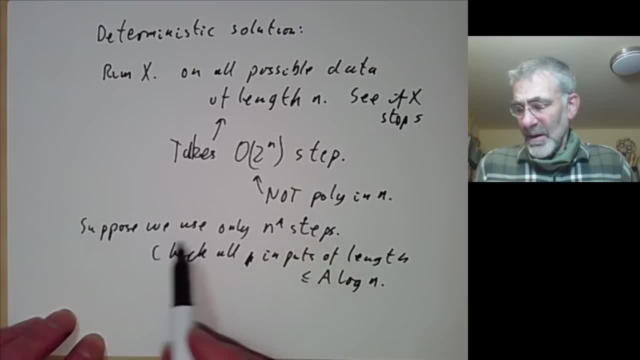 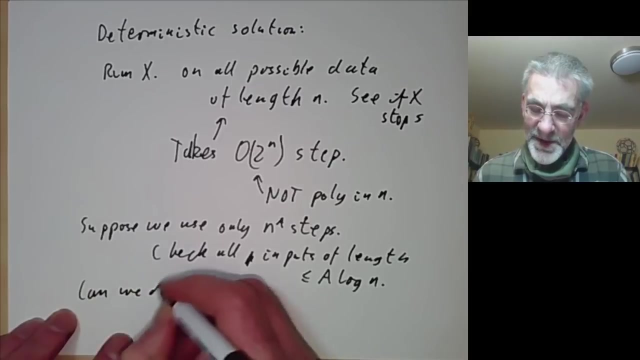 And so what we want to do is find a polynomial way of checking all inputs of length n, And, as we've seen, the obvious polynomial time algorithm only checks inputs of length at most a times log of n. So the problem is: can we do it faster? 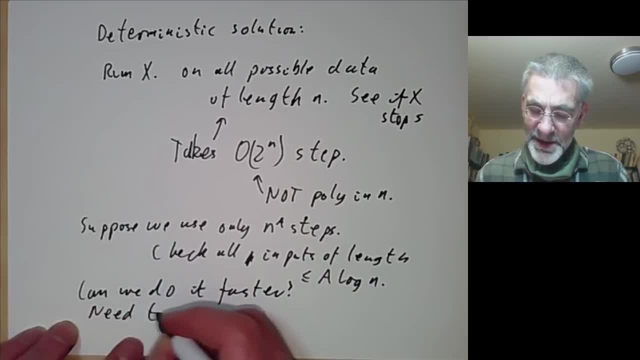 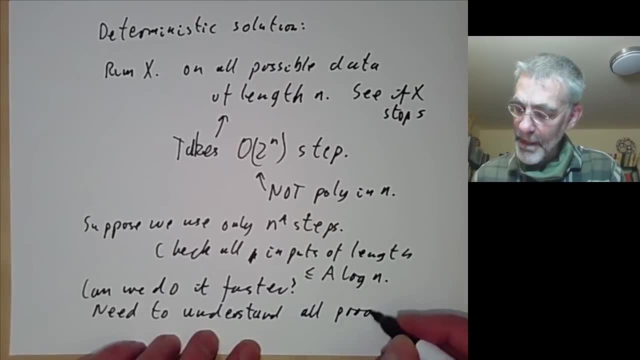 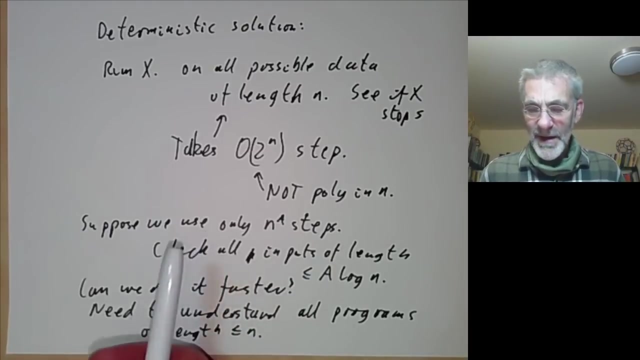 And this seems, in order to do this we need to understand all programs of length less than or equal to n, And we need to understand them well enough to see where they stop in inputs of length n. And this just seems really unlikely because it sort of violates this principle. 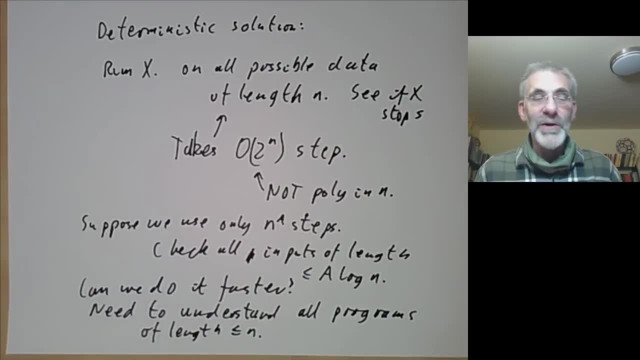 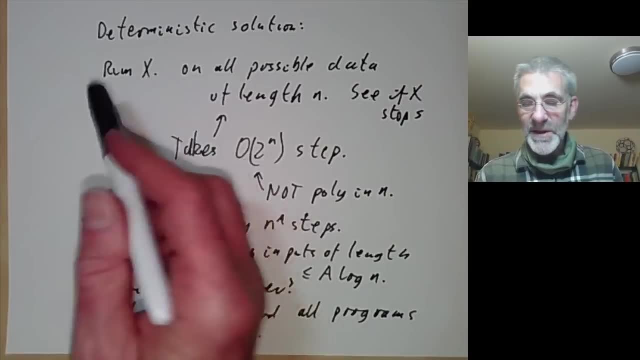 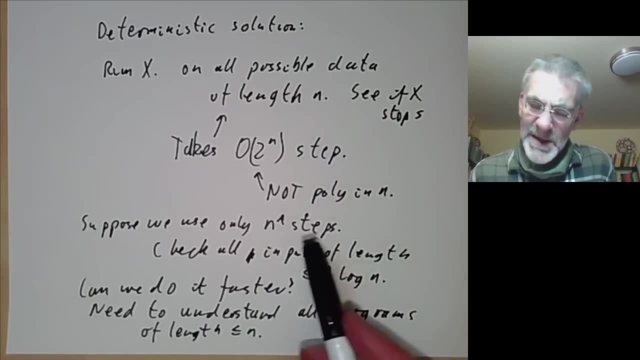 that you can't tell what a general program does except by simulating it. And here we're asking a question about all programs and this strongly suggests we can't tell what they do except by simulating them on all possible input data. And we don't seem to have time. 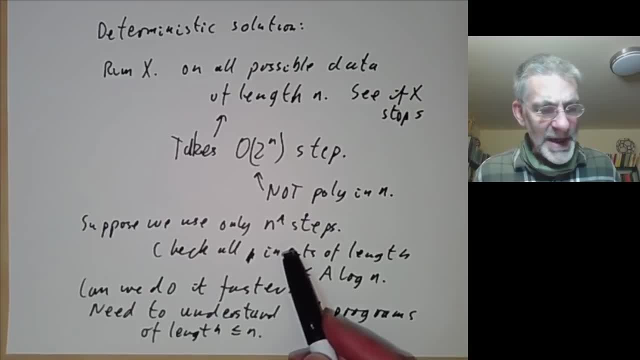 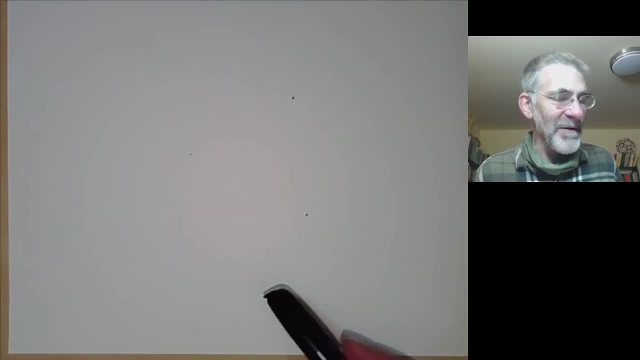 to do this. So this sort of suggests that p is not equal to np. But of course this argument isn't watertight. I mean, I've been waving my hands vigorously at various points in it. So what you can do is: 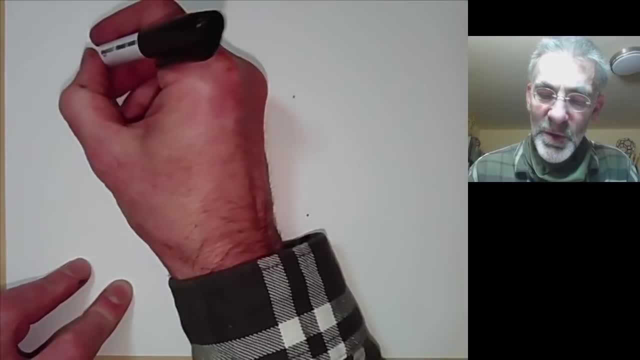 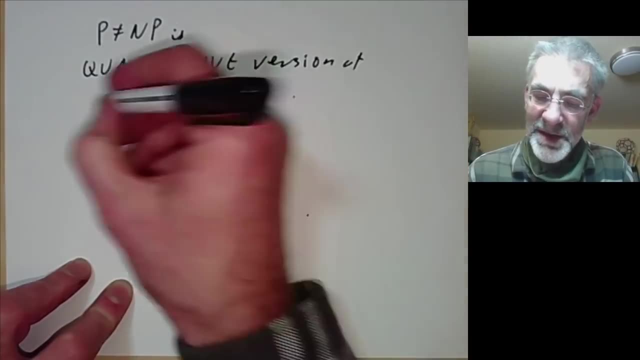 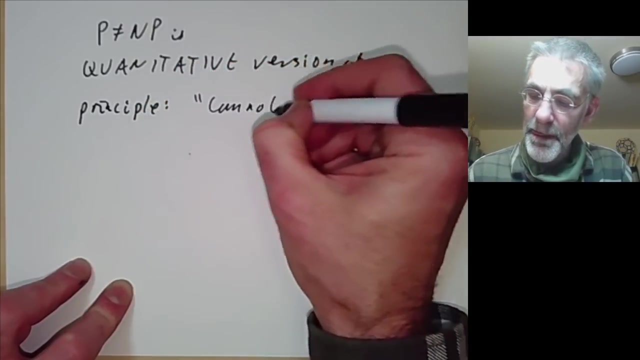 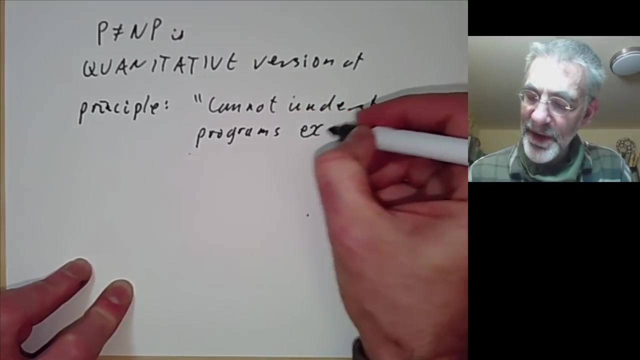 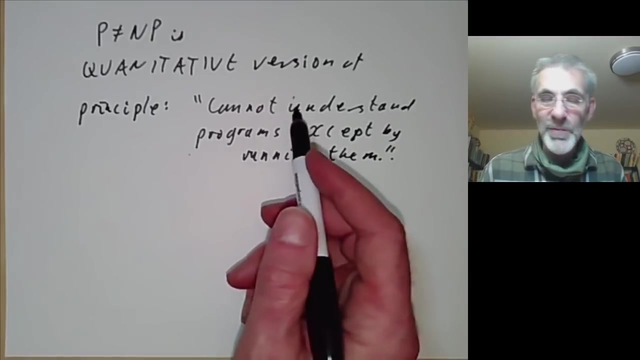 you can say that p not equal to np is a sort of quantitative version of the principle that we cannot understand programs except by running them. So, roughly speaking, if p was equal to np, then we would somehow get some understanding of all programs. on input data. 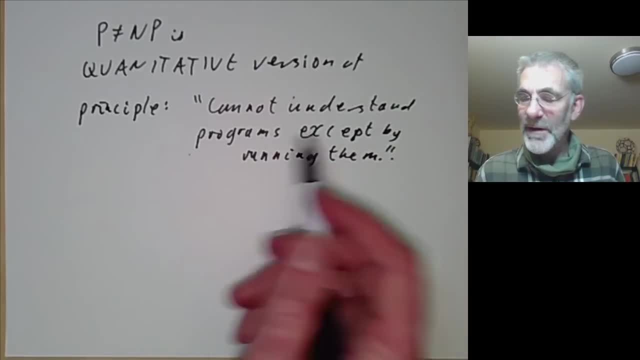 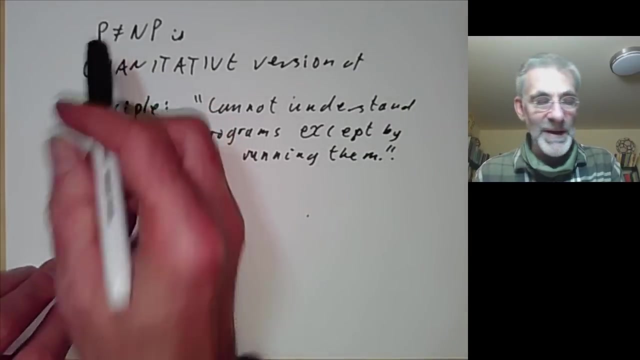 And we would have to do that in a way that was faster than just by running them all on the input data. And, conversely, if we could understand programs without actually running them, then this might give us a way to prove that p was equal to np. 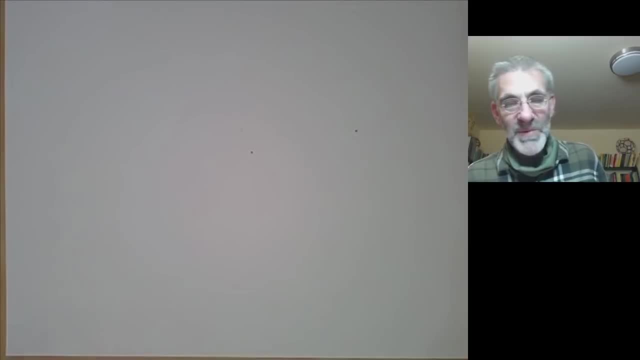 So this seems to me to be quite strong evidence in favour that p is not equal to np, because it's just encoding the well-known fact that it's really hard to understand what a general algorithm does. But there's no easy way to make that argument watertight. 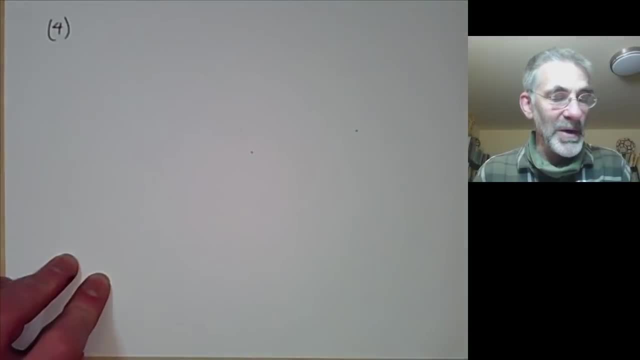 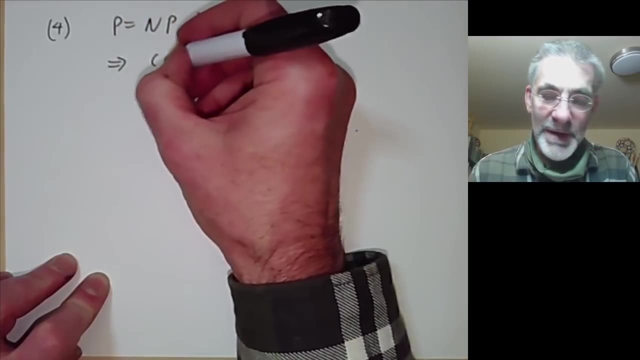 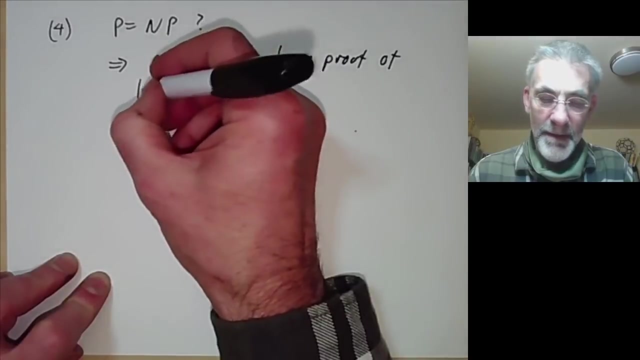 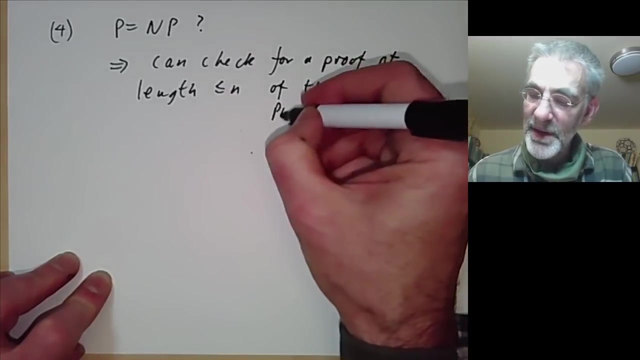 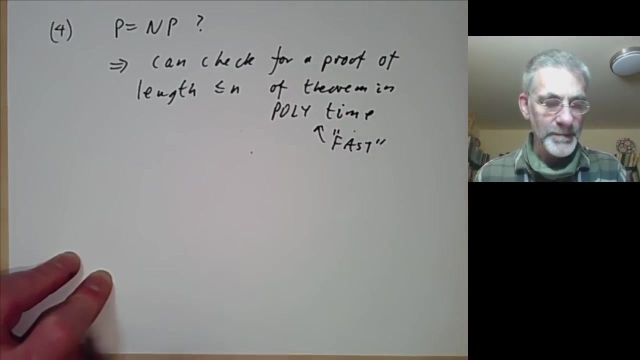 So let's come to argument number four. Suppose p was equal to np. well, this would imply that we can check for a proof of length less than or equal to n of some theorem in polynomial time- And polynomial time is sort of usually fast. Well, this has a rather unfortunate consequence. The consequence is that mathematicians would all be unemployed because our job is to find proofs of theorems, And if there's a fast way of doing this, just by getting your laptop or something to run an algorithm. 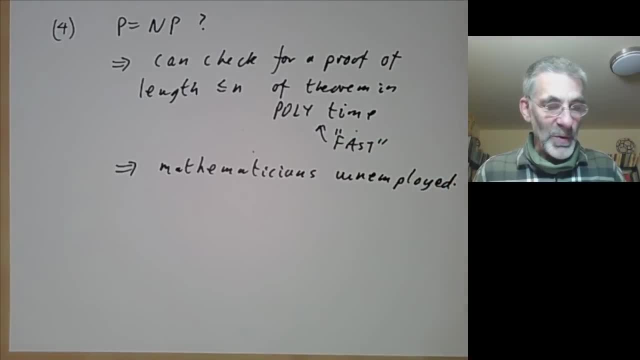 in polynomial time, then we'd all lose our jobs. So this provides well. maybe it's not exactly an argument for why p is not equal to np, but it may be an argument for why we all hope that p is not equal to np. 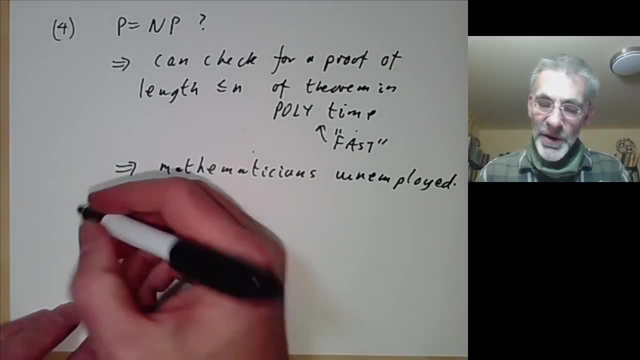 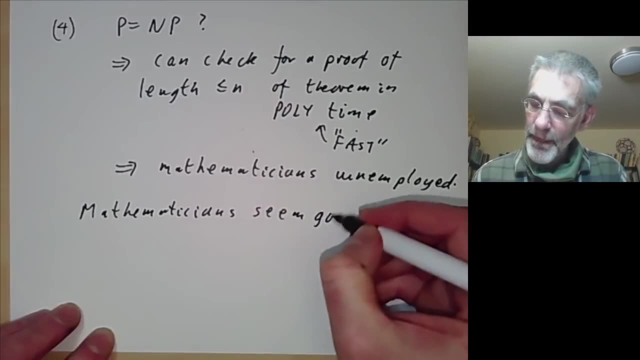 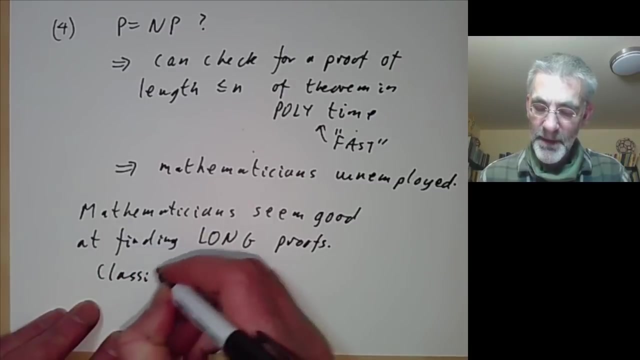 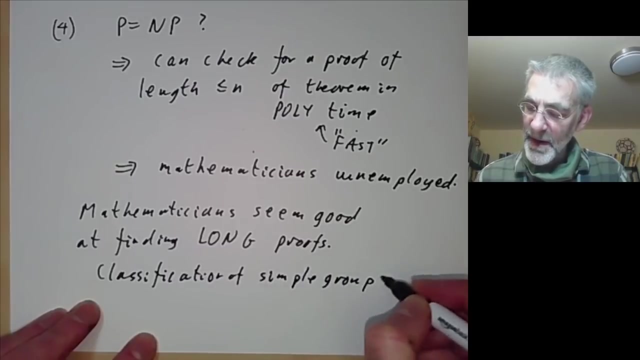 because otherwise we'd all get fired. As a counterargument, mathematicians seem good at finding really long proofs. The most spectacular example of this is the classification of finite symbol groups, And the proof of this is about 20,000 pages long. 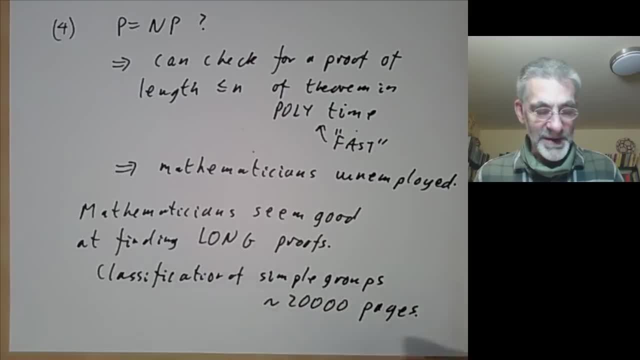 I mean, nobody really knows exactly The proof is spread out so much it's rather hard to tell. So this kind of suggests that in ideal cases mathematicians really are rather good at finding proofs in polynomial time. I mean, we certainly didn't take 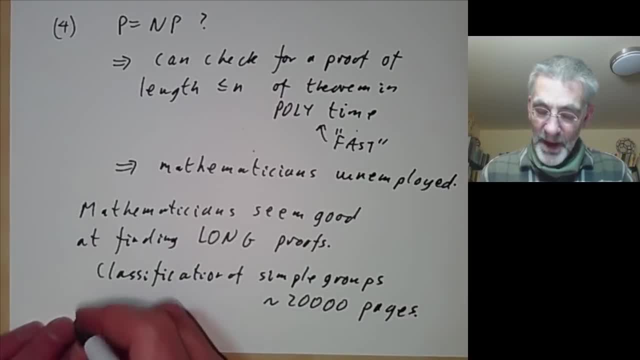 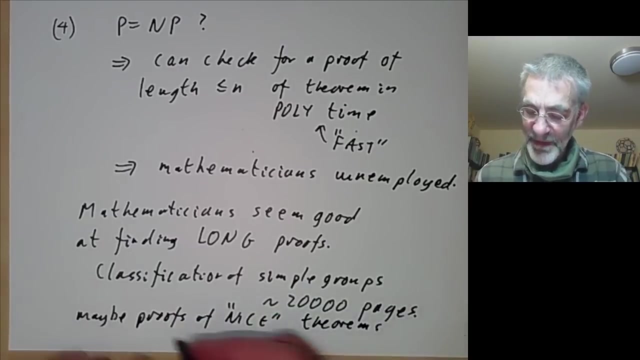 exponential time to find this proof. So it's not clear what's going on. This sort of suggests that maybe proofs of nice theorems can be found in polynomial time, or at least found fast. So you know, mathematics has a lot of nice theorems. 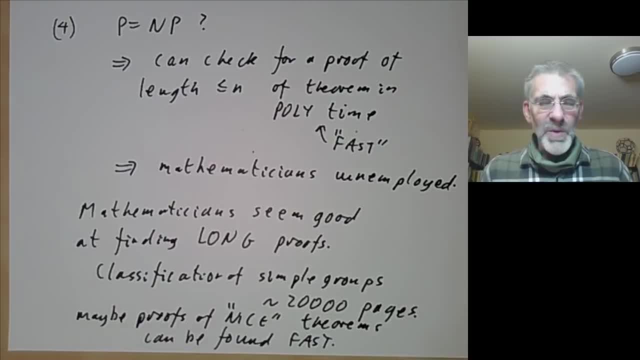 where there's a lot of structure and lots of horrible questions, like this 3x plus 1 problem, where there seems to be very little structure to get hold of And maybe there is, you know, nice theorems. we can find proofs. 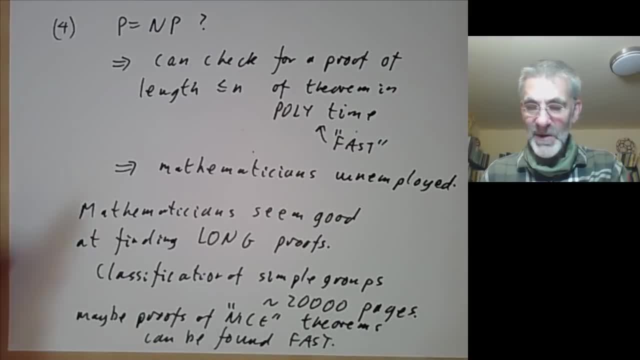 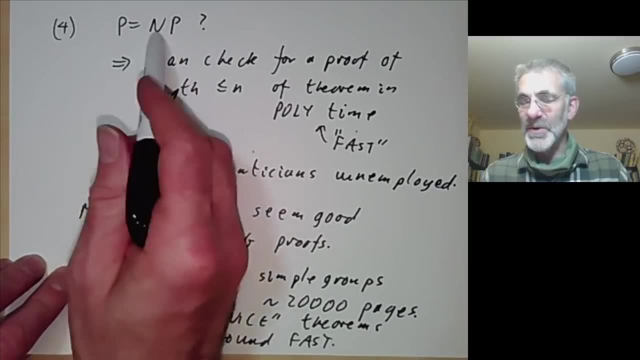 of in polynomial times and nasty theorems. we can't. I don't really know. So argument 4 is sort of really unclear. I would say this slightly: suggests that p is not equal to np, but the fact that we can find long proofs. 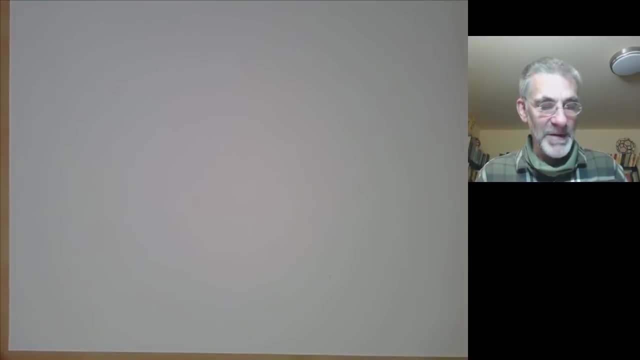 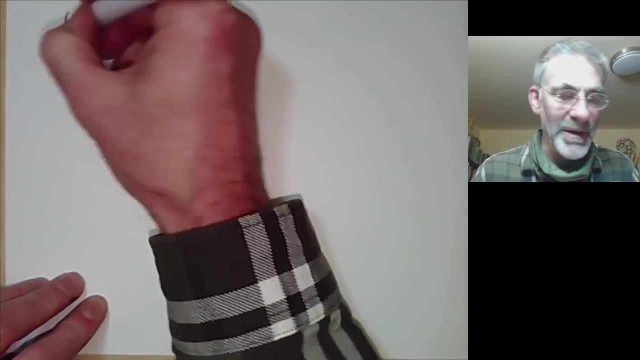 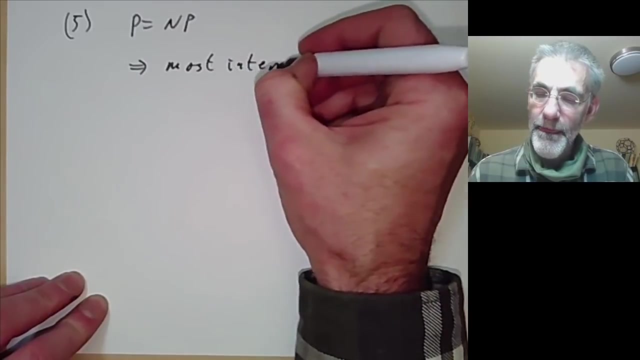 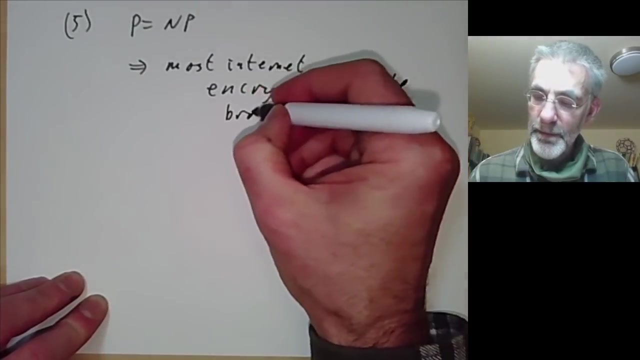 means we should be a little bit hesitant about taking this argument too strongly. So a fifth argument- which is actually similar to argument number 4, is that if p is equal to np, this implies that most internet encryption can be broken. Well, maybe not. 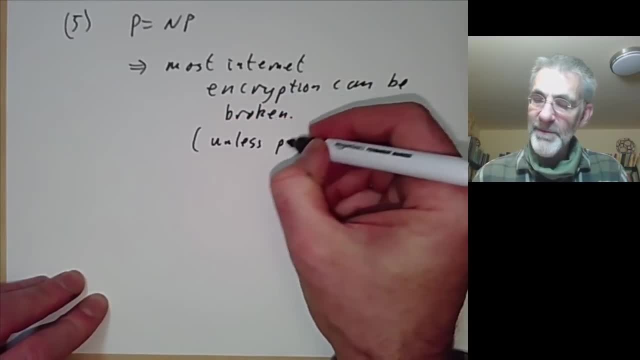 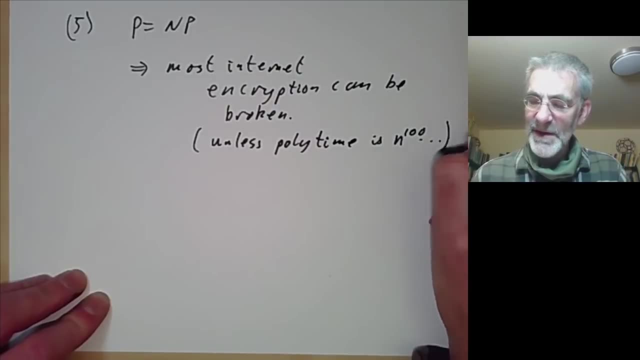 because polynomial time might be really long. So if a polynomial time method for breaking this was, say, n to the hundred or something, then this wouldn't actually be much use for breaking encryption, But an awful lot of the things like the RSA algorithm. 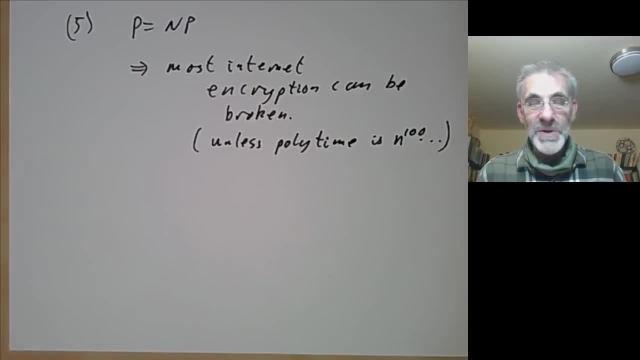 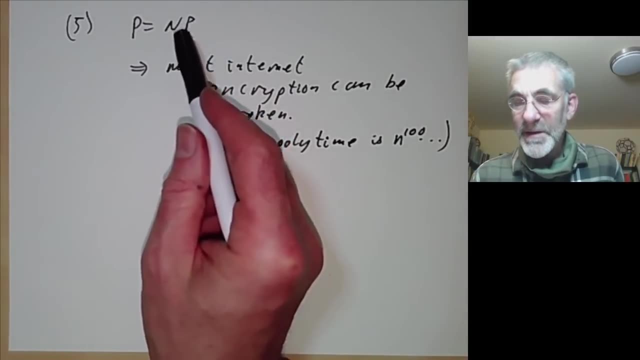 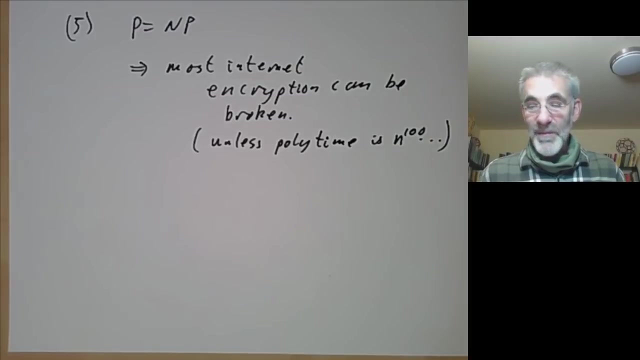 and most other encryption algorithms used on the internet could be broken if we had a fast way of solving non-deterministic polynomial problems. Well, I haven't heard of anybody breaking all encryption on the internet, but it's not quite clear what this proves. 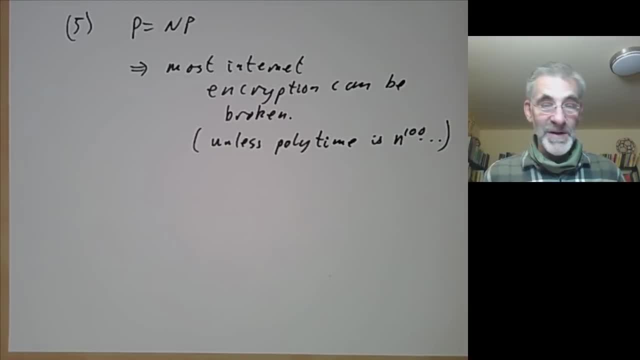 I mean, if someone had figured out how to break encryption on the internet, they'd probably just keep quiet about it and make a huge amount of money. Or if some national intelligence agency had somehow managed to prove that p equals np, it would sit there quietly reading.